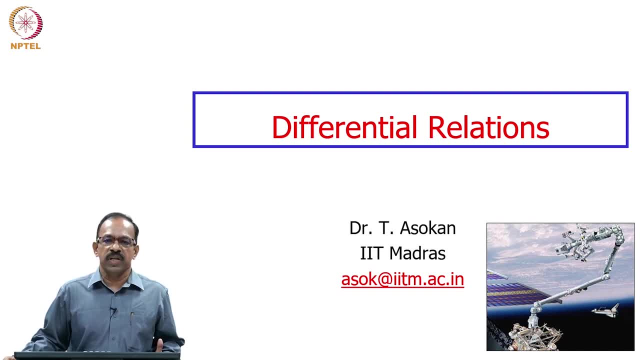 are not only interested in position, but we are interested in the velocity relationship also. For example, if you have a robot and the tool tip is given like this: So you want this to move to this position and that position, we just want this to have a particular velocity. 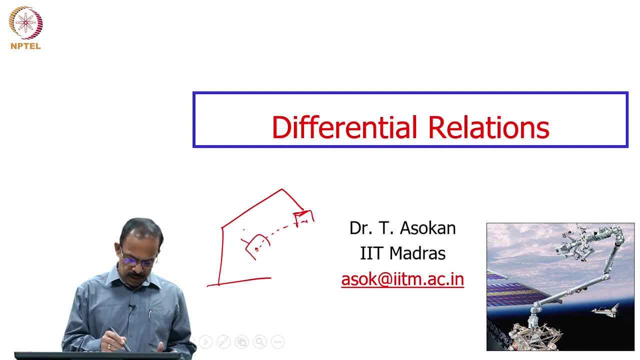 also. So we want this to move from here to here with a particular velocity in the Cartesian space. or we want to say in the tool configuration we want to have a velocity, So we want this to be moved from this position A to B. 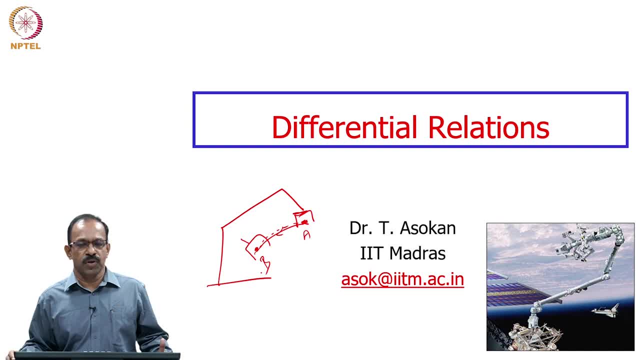 So we want to say, in a particular velocity- either a constant velocity or a velocity profile defined by the user- You want this to move and if that is the case, we need to move the joint also. So these joints also need to have some velocity to get the Cartesian velocity. 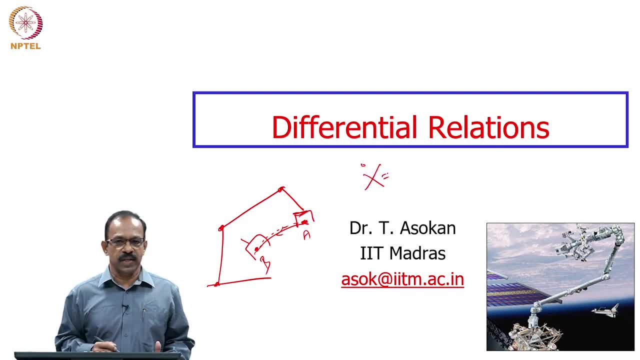 So if you have an x dot, we want to get an x dot, We need to know what is the theta dot corresponding to that and then how can this be related to that? So that is the V 18. Vo 18.. 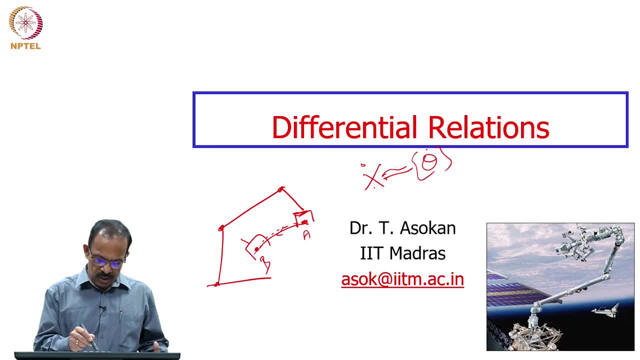 velocity relationship or differential relationship. So how these theta dots, the joint velocity and the Cartesian velocity x dot, are related is known as the differential relationship or differential kinematics. in manipulator kinematics or in the manipulator analysis we call this as the differential kinematics. So we will try to see how we 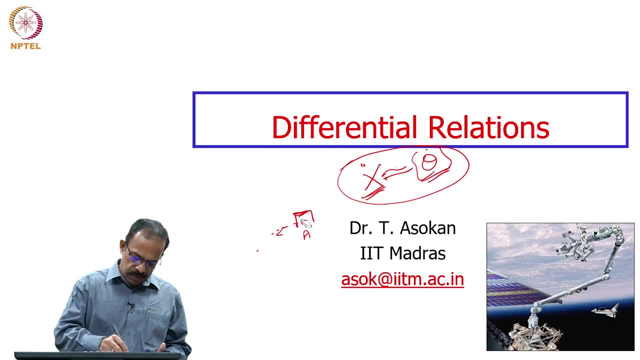 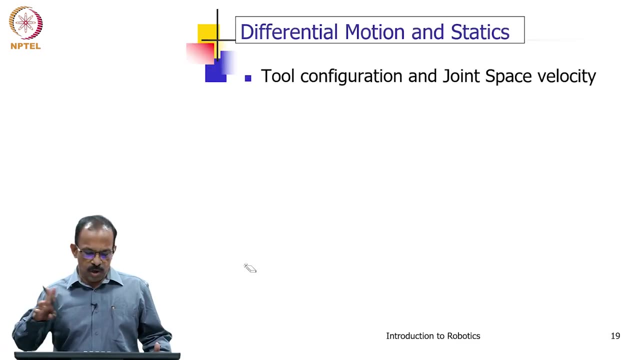 can develop this relationship. once we have the position relationship, how can we convert or derive the differential relationship for manipulator? So that is going to be the discussion we are going to have. So we will talk about the tool configuration and joint space velocity. So joint space velocity is basically the theta dots. 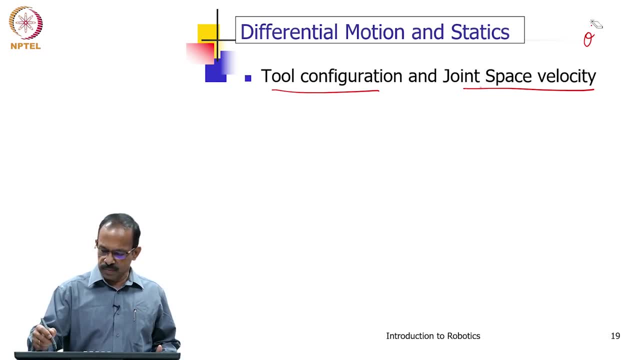 and then the theta dots and tool configuration velocity is the x dots. So you have theta dot and x dots. What is the relationship between theta dot and x dot? is the one which will? that is the tool configuration velocity and joint space velocity. When I say x, it shows that it is the x, y, z, as well as the angular velocities. 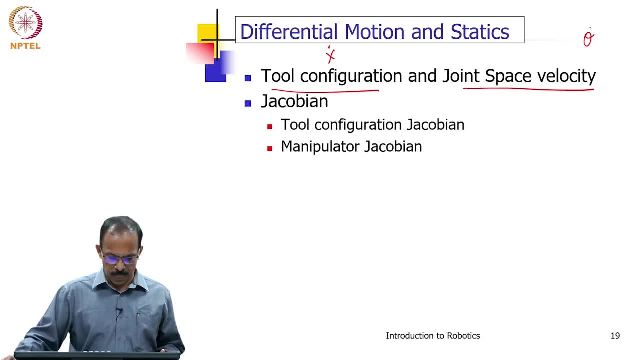 linear and angular velocities in the Cartesian space And we have. when we develop this relationship, we will see that these two are related through a matrix and then that is basically we call this Jacobian of the manipulator or Jacobian matrix. So we will talk about the tool. 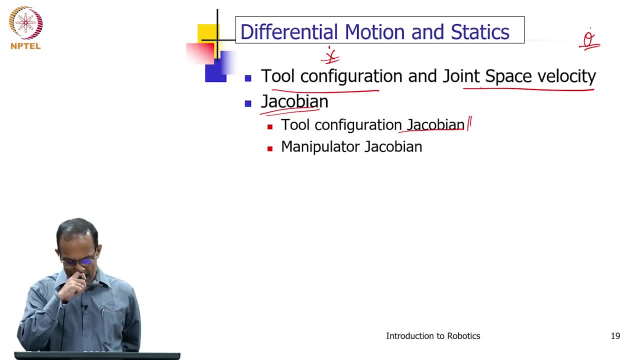 configuration Jacobian as a velocity relationship. and then we can mention that is the manipulator Jacobian, which is the generalized form of this Jacobian, which can be used for other applications also, not only velocity relationship. we can use the is it for the force relationship also? 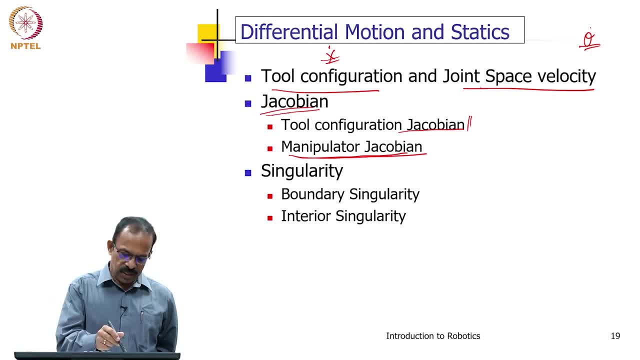 Now, when we go through this and when we know that if you need to get theta dot, x dot from theta dot, we can actually get x dot from theta dot. If you know theta dot, we will be able to get x dot, because theta dot is that you can control, So we will be able to. 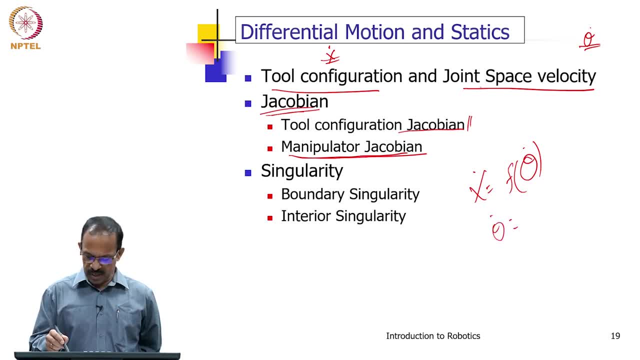 get x dot. The other way is also possible. theta dot can be represented as a function of x dot and we call this as inverse relationship. And when we have this kind of relationship we will see some situations or within the workspace of the manipulator. there may be many points where you 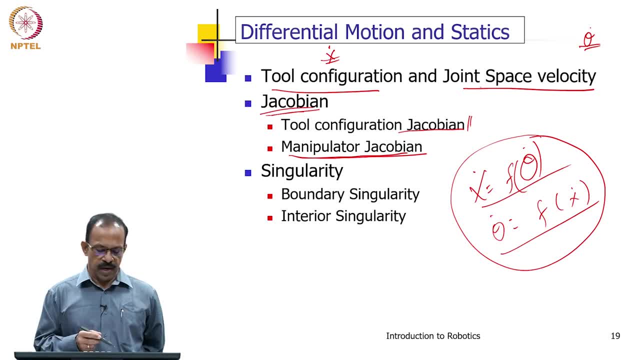 cannot move over manipulator because of some constraints, And that we call it the singularity in the workspace. So we will talk about the singularity and how these actually related to the tool configuration and space, joint space velocity. that also we will try to understand. And then, when we talk about the singularity, there are two times of two types. 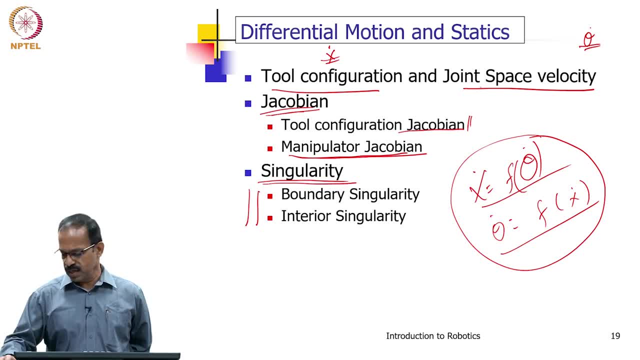 it gives the boundary singularity and the interior singularity which will discuss and we will talk about something called a generalized inverse, because when we try to find out this inverse relationship for the velocity, we will find some difficulty in getting the inverse of a matrix. then we will use something called a generalized inverse. 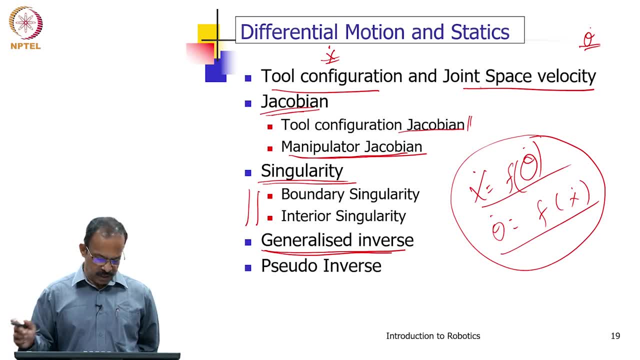 to solve this problem, And finally we will. that is, Euler inverse is one form of the generalized inverse. and finally we will talk about the statics also, where we will be using the relationship that we develop in the differential kinematics to solve for the static analysis. 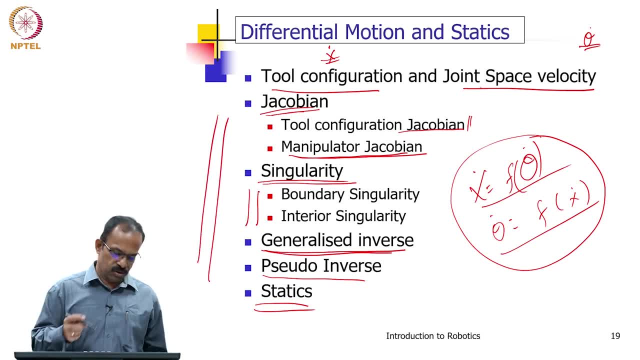 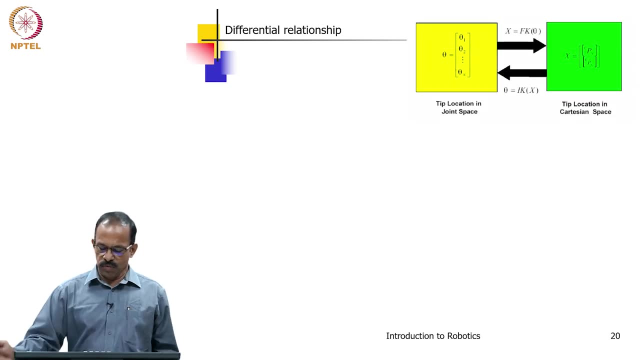 of manipulator. So this is going to be the discussion that we are going to have. Of course, we will solve examples as we discuss in all these topics. So I already mentioned about the differential relationship. So we have theta, that is, a joint parameters or the joint positions, and 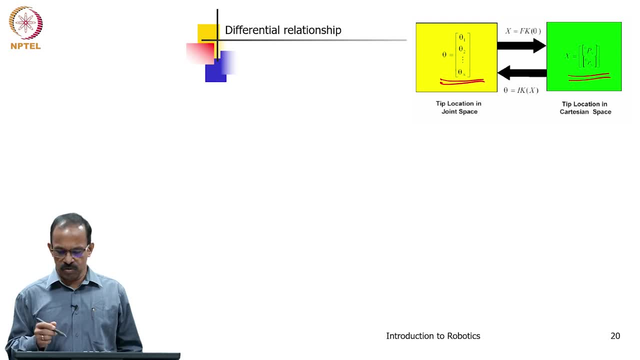 then you have this position of the tool tip, which has got the position vector and the orientation also. So you have the position and orientation of the tool in the Cartesian space- that is known as a tip location in Cartesian space. and then you have the tip location in joint. 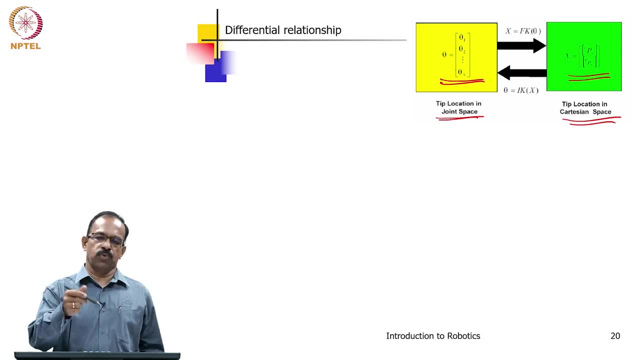 space. So the tip location in joint space is represented by the corresponding joint angles which give you the tip location and, as we know that they are related through the forward kinematics, So f is forward kinematics of theta and theta is the inverse kinematics. 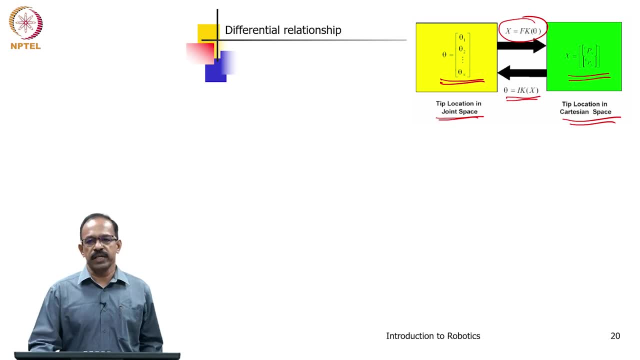 of x. So if you know x, you can apply inverse Kinematics and get the theta, and if you know theta, you will be able to get the x using the forward kinematics. So that is the relationship we have. Now what we are interested in is getting the x dot and theta dots. So the reason why 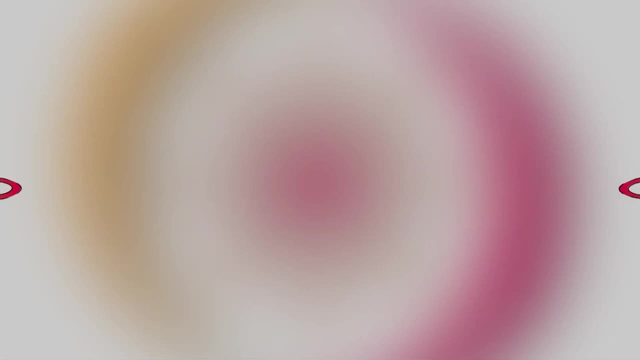 we need to do this to the robot path planning. a problem is formulated: tool configuration space, Because we are interested in the velocity of the tool and most of our problem will be formulated as velocity of tool configuration space. que Mister of our problem will be formulated. 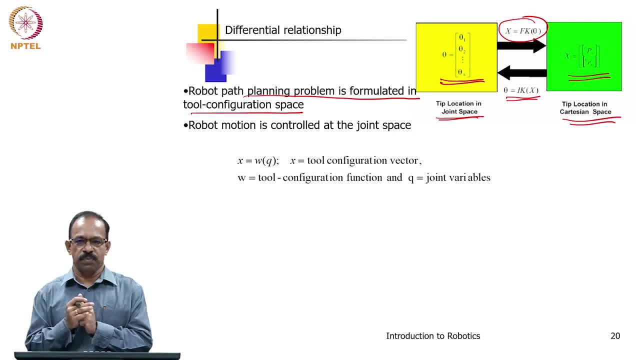 as velocity of tool configuration space, fulfilled by the realistic current sz problem because of tool or the end effector and the robot, motion is controlled at the joint space. So always the motion is controlled at the joint space. we cannot control the tip directly. 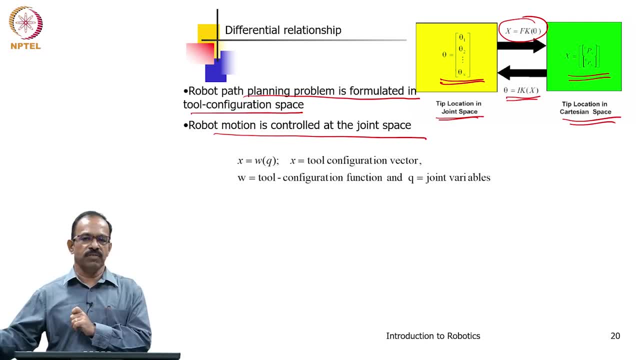 Though we want the tip to have a particular velocity, we cannot command the velocity directly. we need to command the joint velocity So we can control the theta dots, and then we need to get the x dots. So what kind of relationship exists between these two is important, for 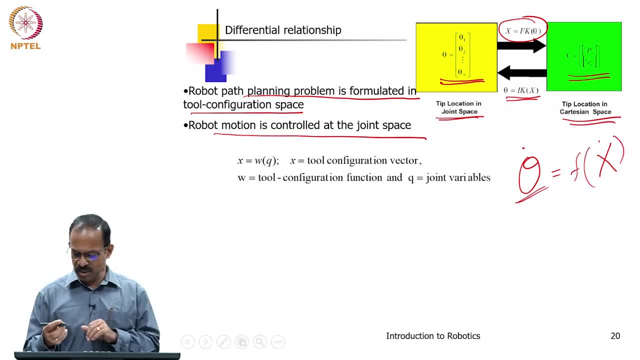 us to command theta dots. So how do we actually command theta dots? to get an x dot or for a given, for a desired x dots? so I have a desired x dot, I have a desired x dot. I want to know what theta dot will give. actually, give me this x dot. 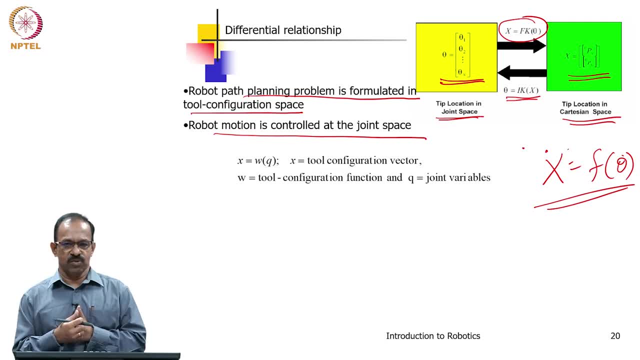 So that is the relationship we are interested, so that I can move theta or move the joint with a particular velocity, so that I will get a desired x dot at the end effector. So this can actually be obtained, as if you reference x as w, q, where w is the relationship between. 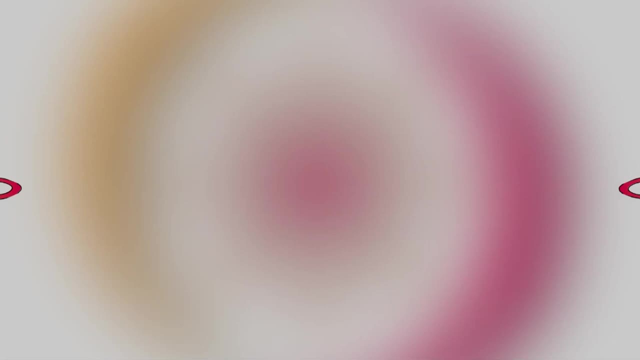 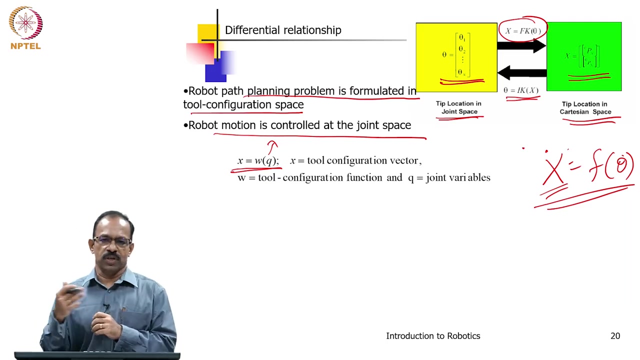 q. q is the joint variable, So we will refer theta in case theta. theta is angle, but we refer q as a joint variable. whether it is theta or d or prismatic or rotary joint, we can use q as the joint variable and then we can say that x is w, q. that is a function. 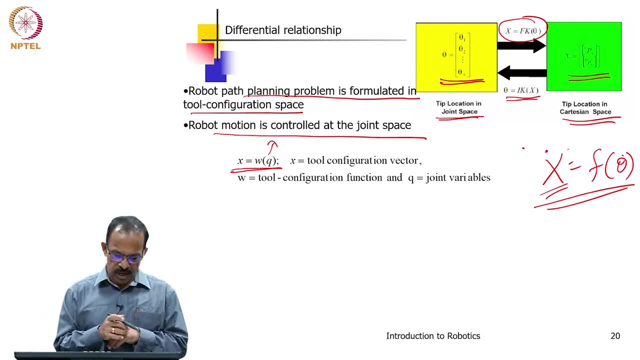 of q instead of fk, we will say that x is w, q, where w is a tool configuration function and q is a joint variable. Now we can actually x dot if you want to write, we will be able to write x dots as a function of q dot and the relation between this x dot and q dot. 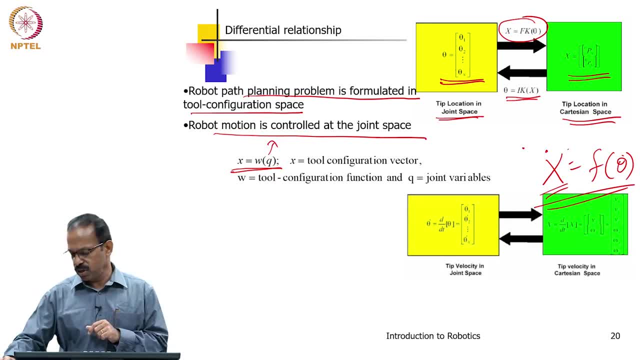 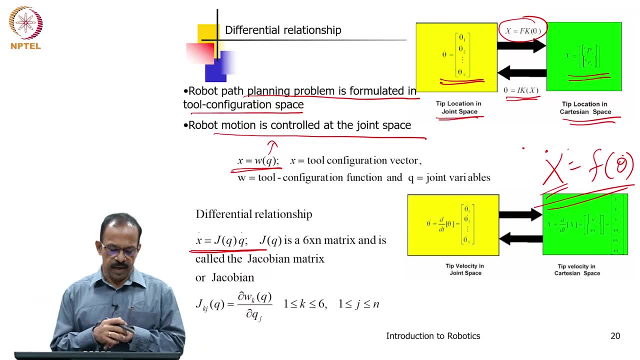 this is a theta dots, theta dot and x dots, So this can be written as: x dot is equal to j q q dot. So we will be able to write this x dot, as the function can be written as j q q dot, where j is known as the Jacobian and it can be obtained by taking the partial. 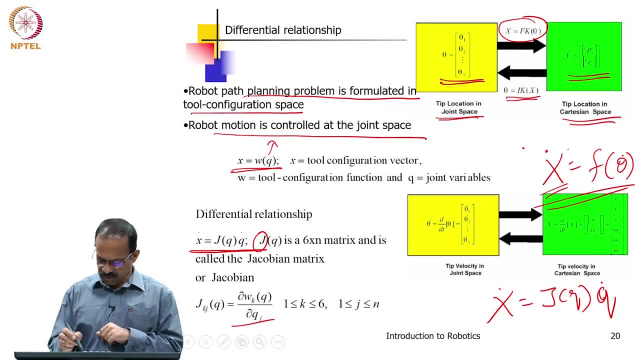 derivative of w with respect to q. So if you have x is w q, so we have x is equal to w q. So we can write it as x dot is equal to partial derivative of w q. So we can write it as x dot is equal to partial derivative of w. 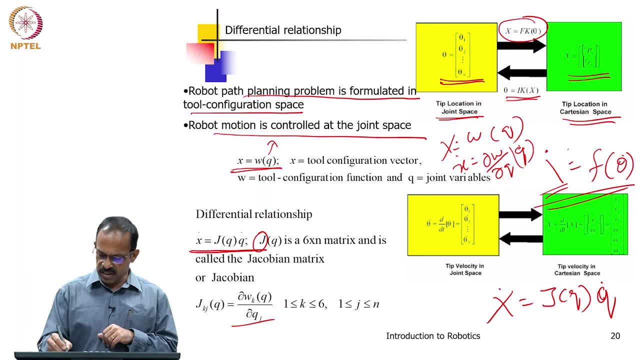 q dot. So that is the relationship that you can get, sorry. So when x is equal to w q, you will be able to write: x dot is equal to partial derivative of w with respect to q q dot. So that is the relationship that you can see. So you will be able to write: x dot is. 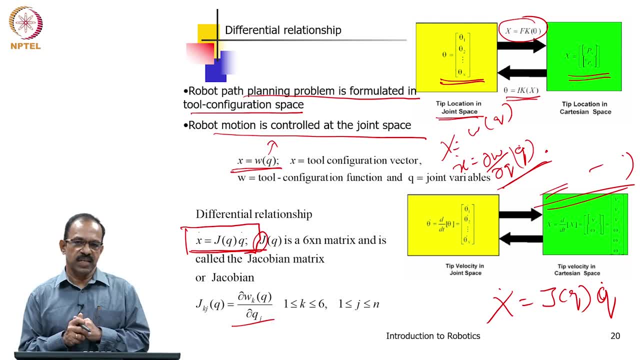 equal to j, q, q dot, where j is the matrix which relates the joint velocity and Cartesian velocity, and this matrix is known as the Jacobian matrix, matrix of the manipulator, or we call it as tool configuration Jacobian because it relates the tool configuration velocity to the joint velocity. so we call it as the tool configuration. 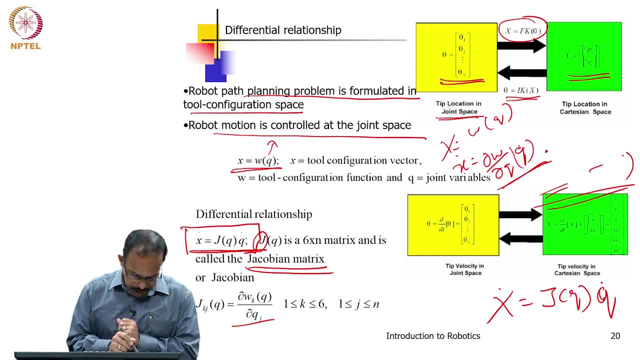 Jacobian And the elements of J. so now J will be a 6 by n matrix, because n is the number of degrees of freedom and we have 3 linear velocity and 3 angular velocity. so this will be 6 and it will be a 6 by n matrix. and this element of J, Jk, Jq, Jk, Jq, is given as partial derivative. 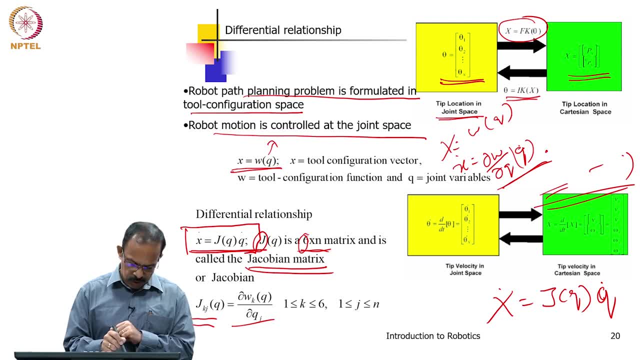 of W, Kq with respect to Qj. so that is basically the elements of Jacobian. So once we have the forward relationship x, w, q, so that is basically the forward kinematic relationship- we can take the partial derivative of that relationship with respect to the joint. 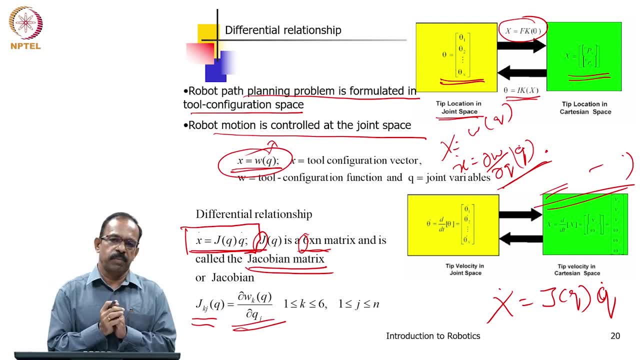 variables And that will give you The Jacobian matrix. and then x dot will be Jacobian multiplied by q dot. So that is the relationship velocity relationship that you can derive from the forward kinematics. So J is the Jacobian which relates the tool configuration velocity to the joint velocity. 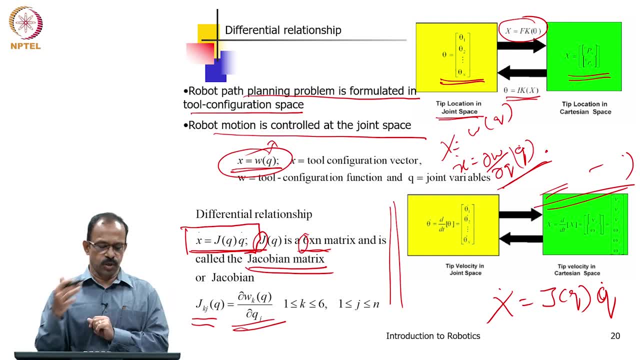 So this is the relationship: x dot is J, q dot. so if you know q dot you can actually get x dot by simply multiplying q dot with J. so that is Jacobian. So K is 1 to 6 and then J is 1 to n. n is the number of degrees of freedom. 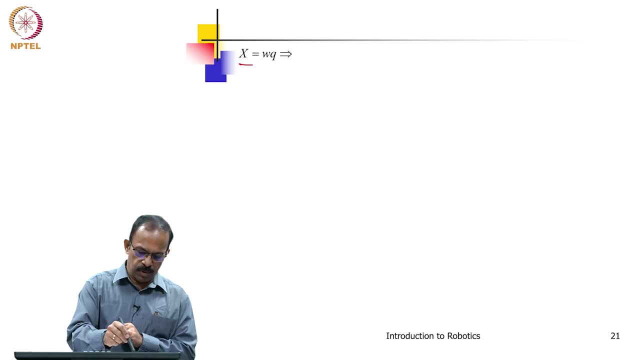 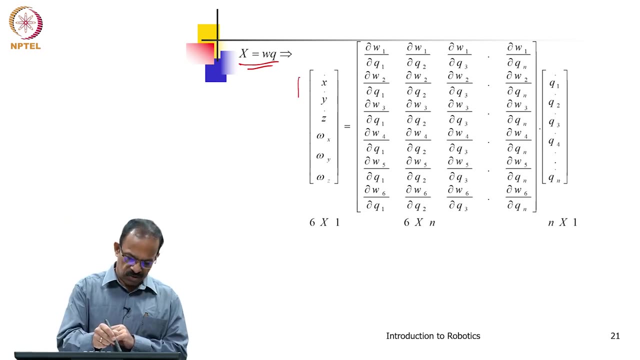 So this can be written in the matrix form as like this: So if x is Wq, we will be able to write down the J elements as like this: So you have this x dot as x dot, y dot and z dot. These are the x dot, y dot, z dot. 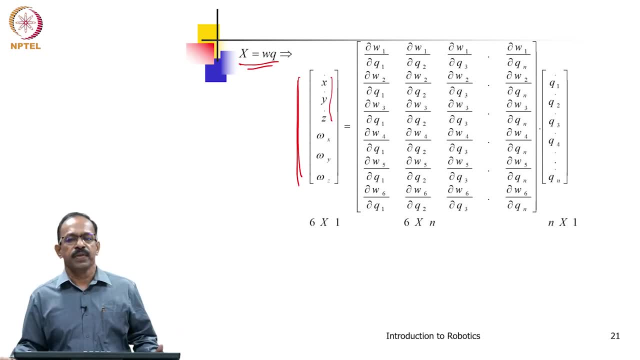 So you can write down the j elements as like this: So you have this x dot as x dot, y dot and z dot. These are the x dot, y dot and z dot. So you have these three linear velocities in x direction, y direction and z direction. 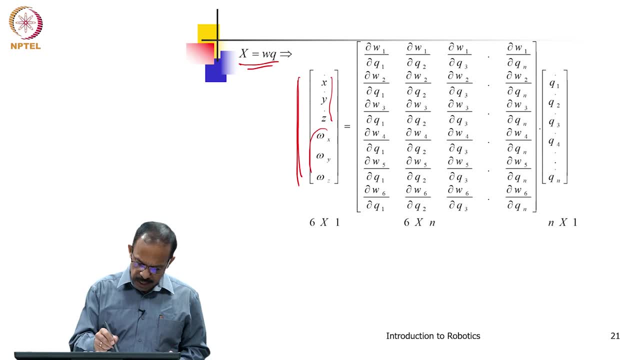 in Cartesian space. and then you have this omega x, omega y, omega z, which is the angular velocity with respect to x, y and j axis. So these are the three linear and three angular velocities. and then you get this element by taking the partial derivative of W1 with respect to q1, q2 to qn. so W1 is the relationship. 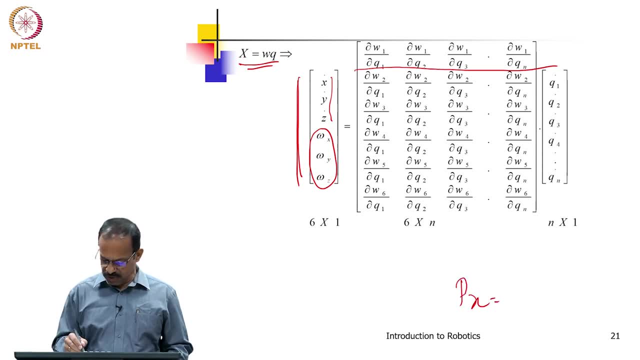 for x. Px is a function of. we write only the position of x. we know it is a function of q, So we consider this as W1 as the function. we write it as W1q. Then you take partial derivative of W1 with respect to q1, q2, q3, qn. you will get the 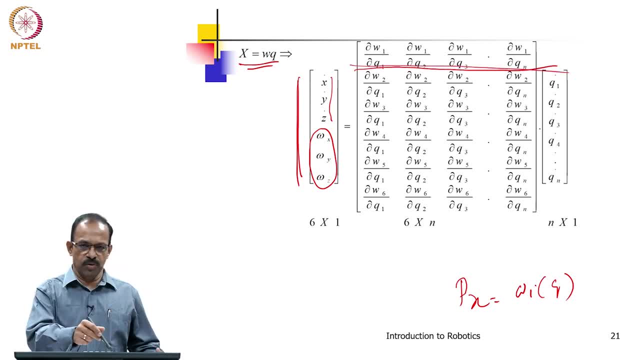 first row of the Jacobian, that is for the x velocity And for y velocity. you take the second relationship, Py relationship. so you will be having n relation, for Py is equal to W1.. Okay, W2q. then you take the partial derivative of this W2 with respect to q1, q2, etc. 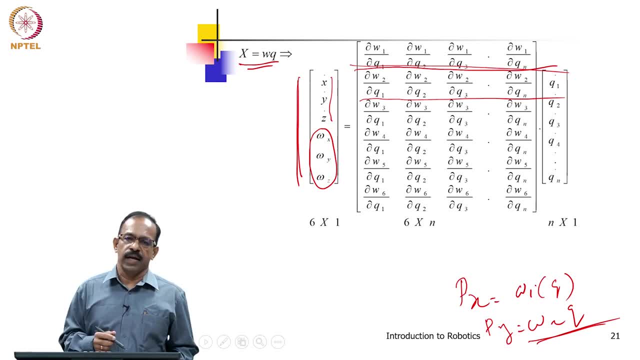 So this is the way how you will get the Jacobian elements, the elements of the Jacobian matrix. Now you can see this. this is a 6 by 1 vector- three linear velocity and three angular velocity- and this is an n by 1 vector because you have n joints and therefore there will be n joint. 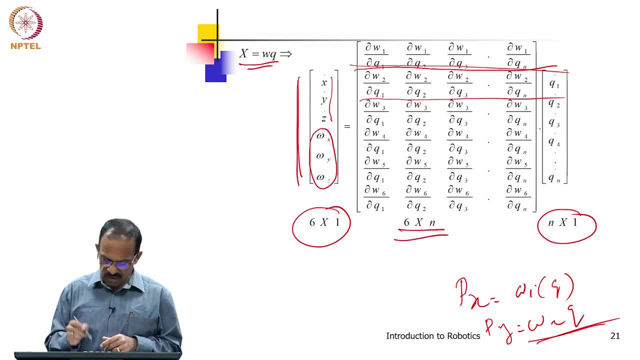 velocities. So it is a n by 1 vector and then this will be a 6 by n vector. So it will be a 6 by n matrix. So it need not be a square matrix, it will be Jacobian, will be a matrix, depending on. 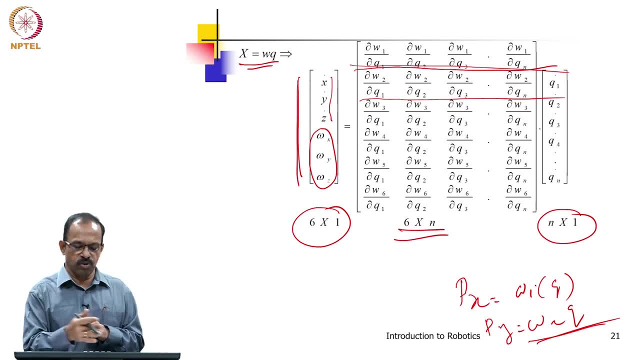 the dimension of n. depending on the n, the dimension of matrix will be 6 by n. So for a 7 degree of freedom, it will be 6 by 7, for a 5 degree of freedom, it will be 6 by 5, for a 6 degree of freedom, it will be a 6 by 6 matrix. 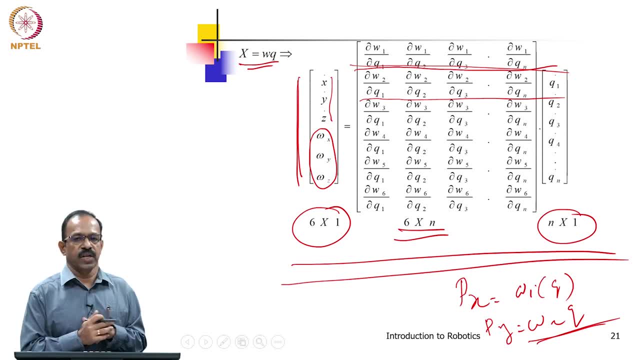 So this is the Jacobian, how you get the Jacobian. So we will take few examples to see how the Jacobian can be developed. Okay, Thank you. My first example should be this: So we will take this x dot for any manipulator. 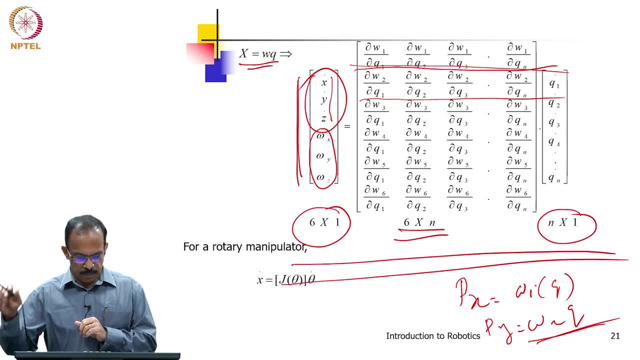 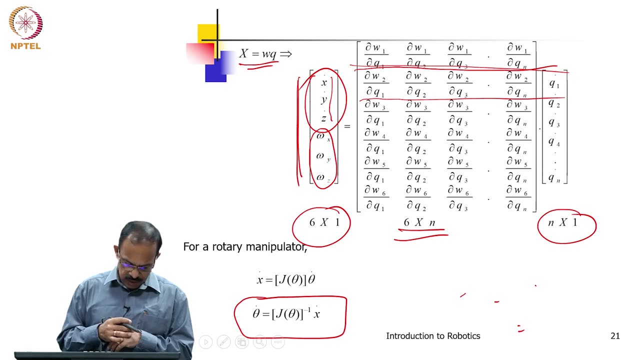 So first we look only the linear velocity part and then later on I will explain how the angular velocity can be calculated. angular velocity part can be calculated. Okay, So for the rotary manipulator it will be j, theta, theta, dot, And you can actually get the inverse also. 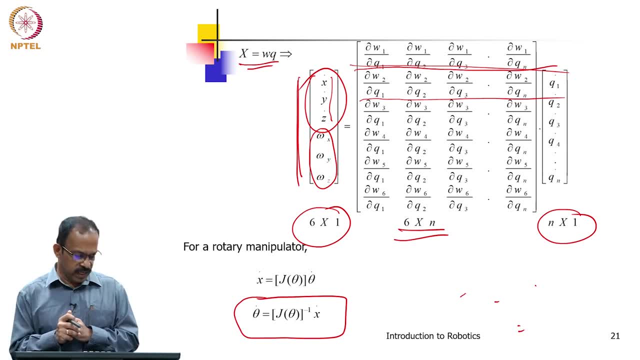 x dot known, then we can get the theta dots. So if theta dot, that is, the joint velocities, are known, we can easily calculate the x dots using the j, theta, theta dots. Now the other case: if you are, you have you know what is the Cartesian velocity you want. 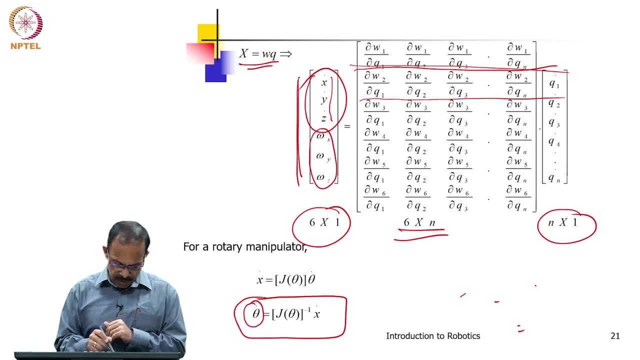 to find out the corresponding theta dots For a given x dot. what is the theta dot? can be obtained by getting the inverse of Jacobian. we take the j inverse x dot. So in the workspace, suppose you have the workspace, this is the workspace and you want this to move from here. 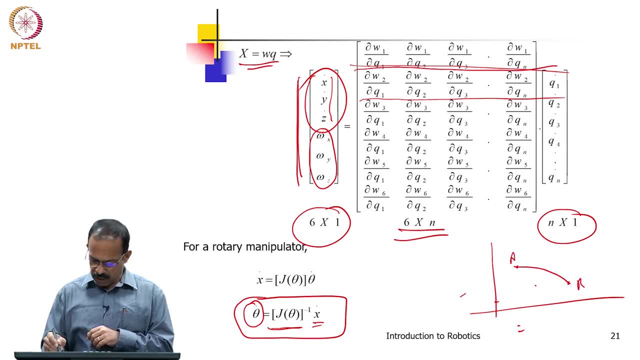 to here: a to b in the workspace. you can specify what is the velocity. you want this, want this tooltip to move from a to b. If you can specify the velocity, we can find out what is the corresponding joint angles, velocity, joint velocities, using this relationship. 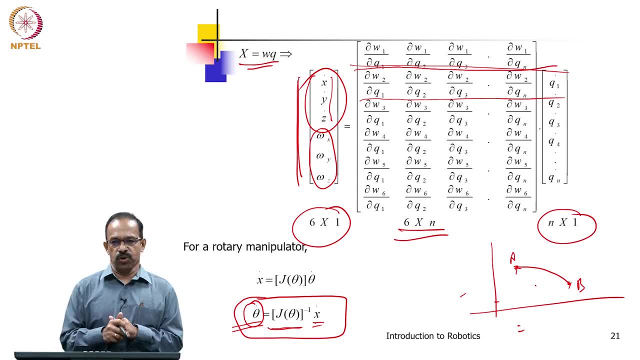 j inverse x dot. so that is the inverse relationship for the velocity. So x dot is j theta dot and theta dot is j inverse x dot. So the, though it is a direct problem of getting theta dot and x dot, it actually creates a 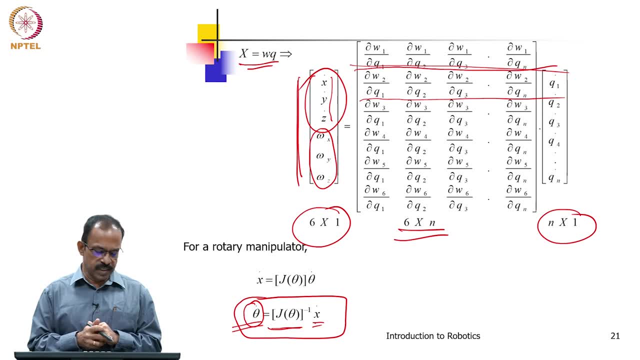 lot of issues when we start computing the theta dot for a corresponding x dots. We will be discussing that. So these are the issues. but one issue is that the j theta inverse, so we have to get an inverse of j And one problem, immediate problem, is that when it is non-square matrix, 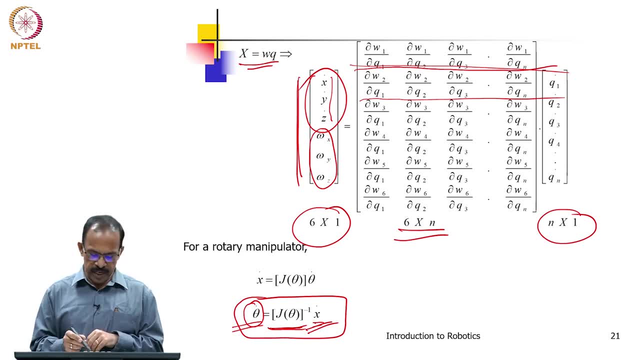 how do you take the inverse? So 5 degree of freedom robot for a 5 degree of freedom robot, this will be a 6 by 5 matrix. And how do you get the inverse of a 6 by 5 matrix? 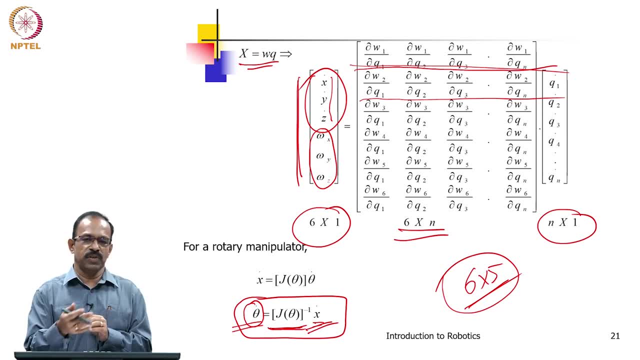 And we know that the inverse need to be. to calculate the inverse, we have to have a square matrix And then only we will be able to get the inverse. But in this case, when it is 6 by 5, what we will do? does it mean that for this relationship is applicable only for the 6 degree of freedom? 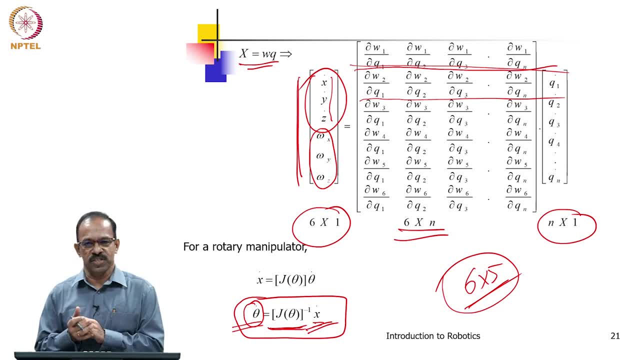 robot or other robot also can actually use the same relationship. So that is one immediate problem. And another problem is that this j, even if it is a square matrix, as you know, not all matrices can be inverted, Again, depending on the type of the matrix and its properties. 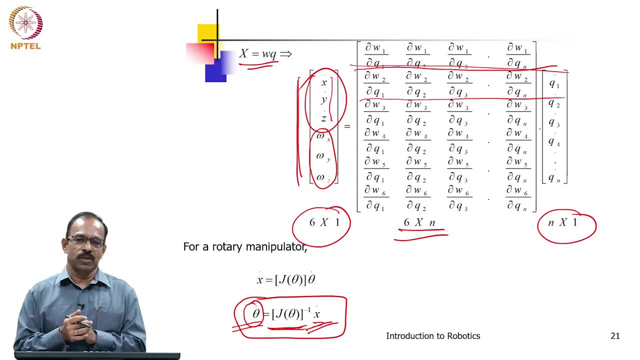 you may find sometimes that there cannot be inverted because of its rank, its rank is not equal or there is some problem with the matrix condition number. then you would not be able to get the inverse. So these are the two major problems that we will face when 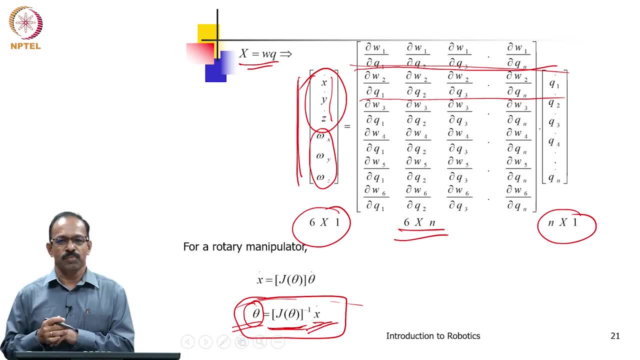 we go for the calculation of theta dot from x dot. So we will discuss that issue later. So first let us see: how do we get the j for a manipulator. how do we first calculate the Jacobian for a manipulator? we will see then, later on we will discuss about the problems. 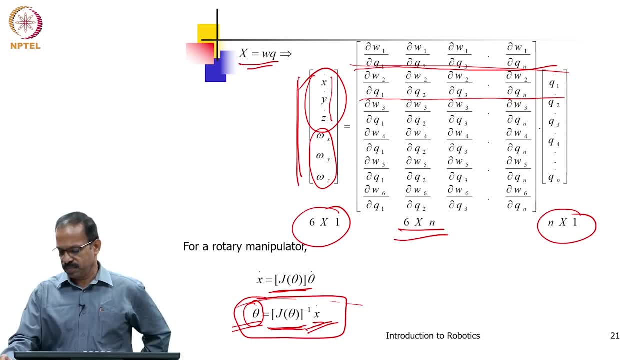 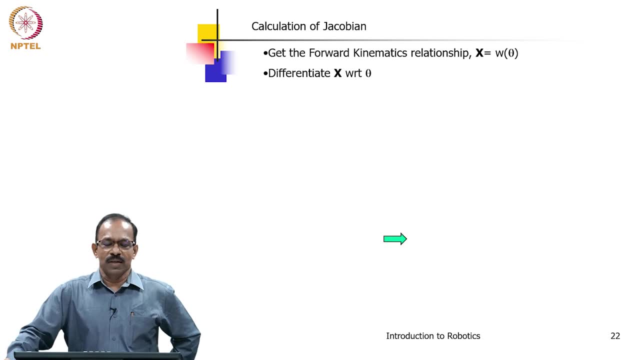 associated with the inverting of Jacobian. We will take a very simple example initially to see how to how to calculate the Jacobian. So we know that it is differentiation with respect to theta. so we will take a very simple manipulator of a 1 degree of freedom. so we will take a 1 degree of freedom, single link. 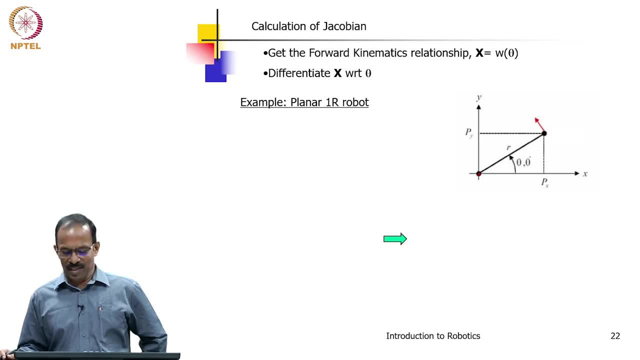 manipulator, planar manipulator, to make it very simple. so we will. we know that this is the P. I mean, this is the tip and this is theta. So you have only 1 degree of freedom so we can easily write Px and Py. so Px is equal to something and Py is equal to something. 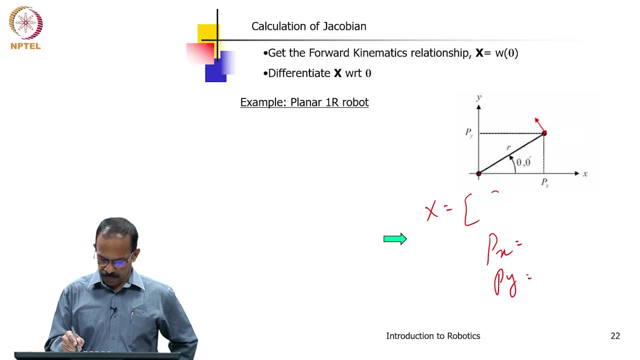 So that will give x is equal to something, to something multiplied by theta dot, I mean theta. this is so we will be able to write x. dot is something multiplied by theta dot and this elements are basically you will get that is, partial derivative of Px with respect to theta and partial derivative of Py with 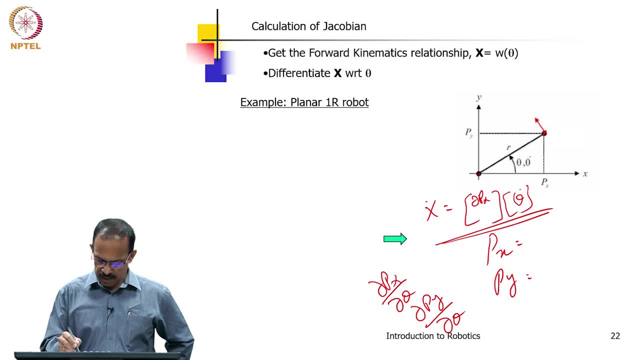 respect to theta. so that will be the element here: partial derivative of x and partial derivative of y theta. So this will be the two elements in this case and, as you know, it is only x dot and of course x dot means x dot and y dot, in this case Px dot, Py dot. so this is the way how. 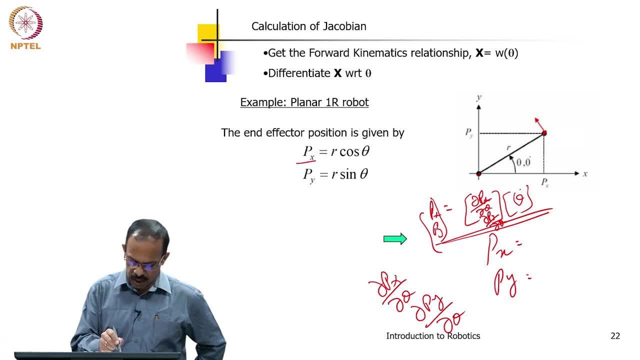 we can actually get it now if I do this. we know that Px is equal to r cos theta, Py is equal to r sin theta. and then to get the Jacobian, we take the partial derivative and find out what is the Jacobian that you are getting. 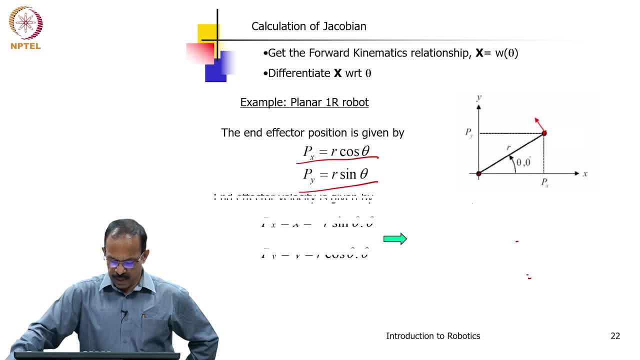 So take the partial derivative of Px with respect to theta. It will be minus r sin theta theta dot. Px, dot will be minus r sin theta theta dot and Py will be r cos theta theta dot. Now if you write it as a matrix, we will get it as x dot y dot. when I say x dot, y dot, Px. 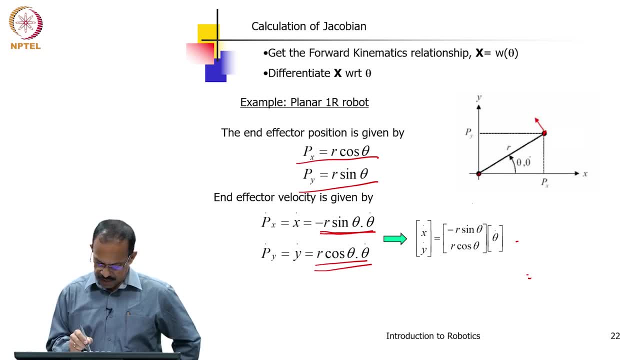 dot, Py dot is minus r sin theta r cos theta, theta dot. so that is the relationship. get, and this is the Jacobian for the single degree of freedom manipulator, it is minus r sin theta r cos theta. So you are talking only about Jacobian. 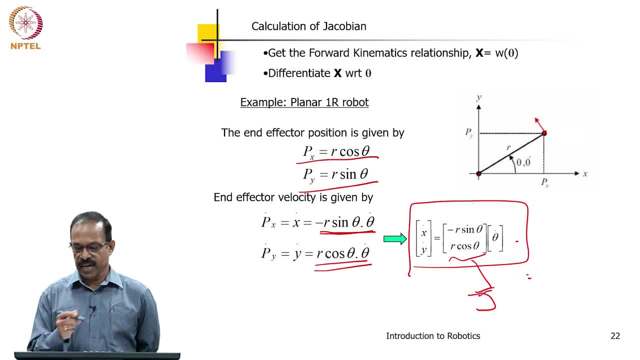 You are talking about the linear velocity for the time being. we will discuss angular velocity later. So this is the x dot and y dot for this manipulator. So this is the principle to be followed, whether it is a 6 degree of freedom or a 7 degree. 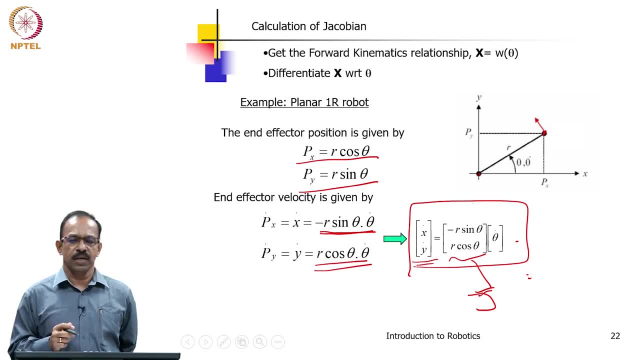 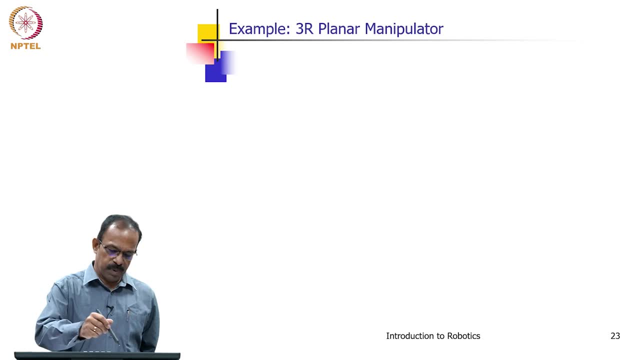 of freedom. we will follow the same principle and then start calculating the Jacobian. that is what we do in this case. So let us take the 3 r planar manipulator. again, it is only planar, we are talking about it. We will see how can we get the Jacobian. 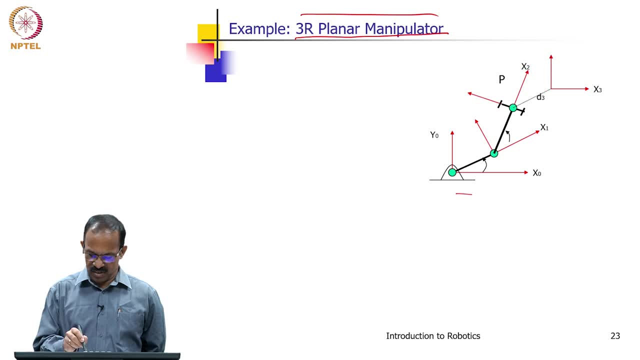 So look at this. So this is the planar manipulator which we already discussed during the forward and inverse kinematic analysis. So we know what is Px and Py and Pz also we know. So we have the relationship for Px, Py, Pz because if this is taken as L1, L2 and theta, 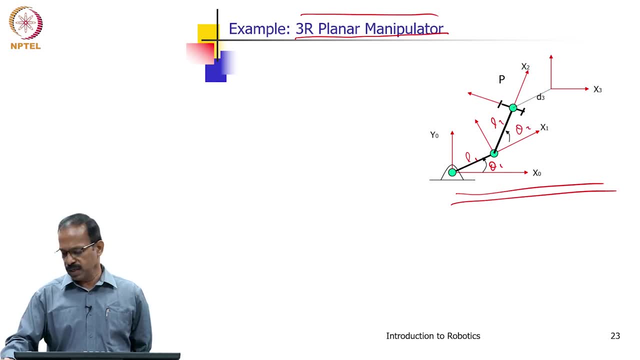 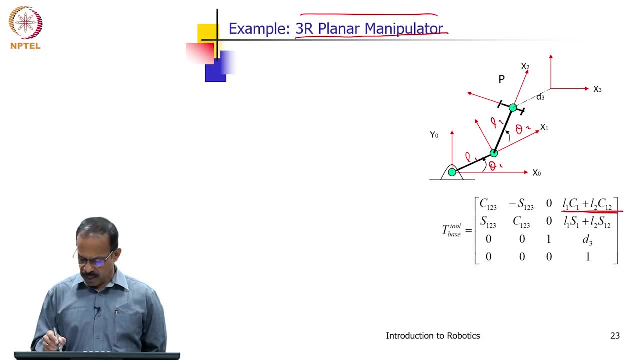 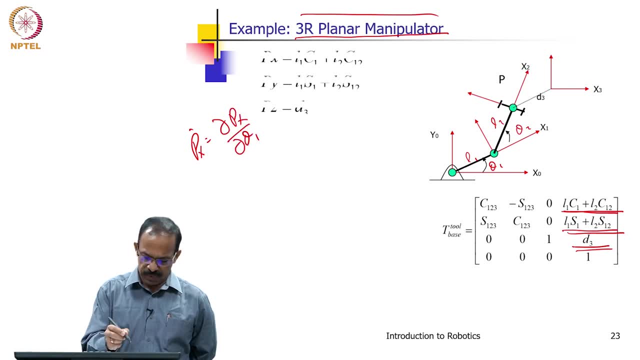 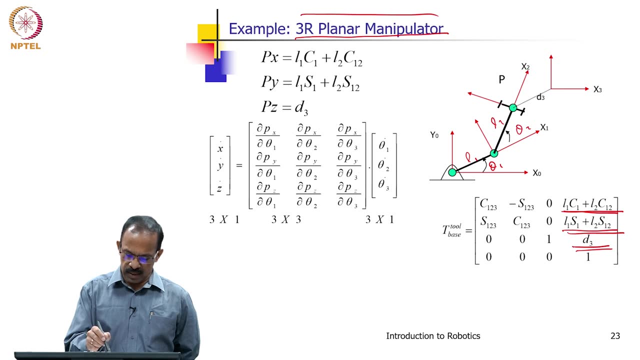 partial derivative of Px with respect to theta 1, and so if you write it like this, we will get it as x. dot is Px with respect to theta 1, theta 2 and theta 3, and Pz theta 1, theta 2, theta 3.. 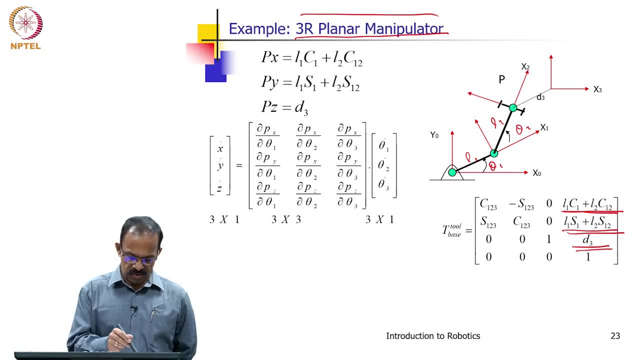 So that is the way how we get x dot, y dot and z dot. So you can see this is a 3 by 1 vector, 3 by 3 matrix and it is a 3 by 1 vector. Now we take Px with respect to theta: 1 is L1, C1 plus L2, C1, 2.. 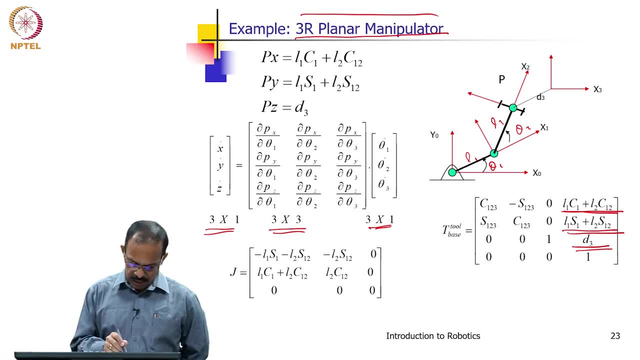 So we will be getting this as minus L1 S1, minus L2 S1 2, and this would be minus L2 S1 2, and this is L1 C1 plus L2 C1 2, L2 C1 2, and this would be 0 because Px with respect to. 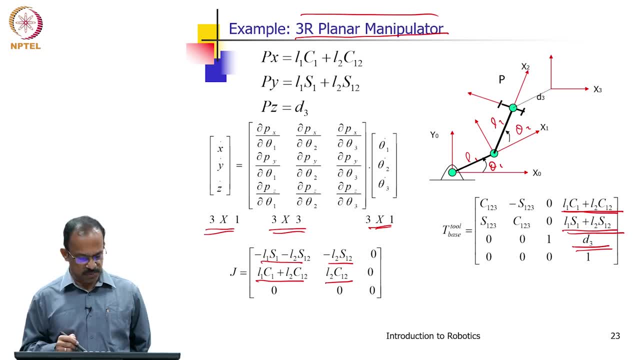 theta 3.. So this will be the Jacobian for the linear part: linear velocity of the manipulator. So this is how you can get the Jacobian for manipulators. So whether it is a 3 degree of freedom or a 5 degree of freedom, use the same principle. 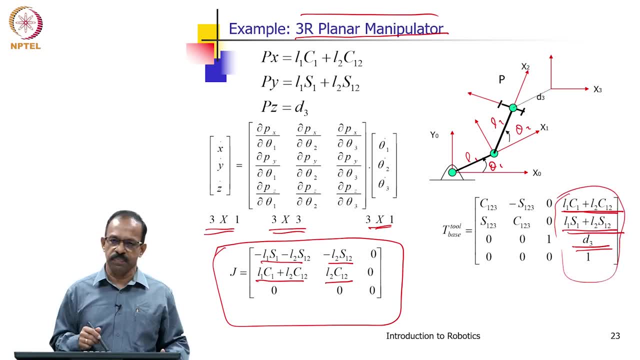 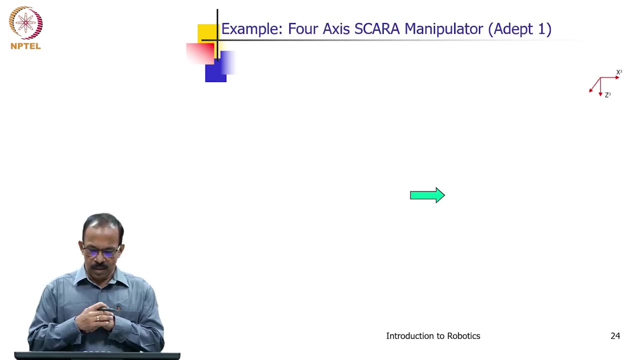 because get the relationship from your forward kinematics Px relationship or x relationship and then get the, take the partial derivative. Take the partial derivative, get the matrix, so you will be getting the Jacobian for this manipulator. This is another example, again a four axis manipulator. it is a Scara manipulator. four. 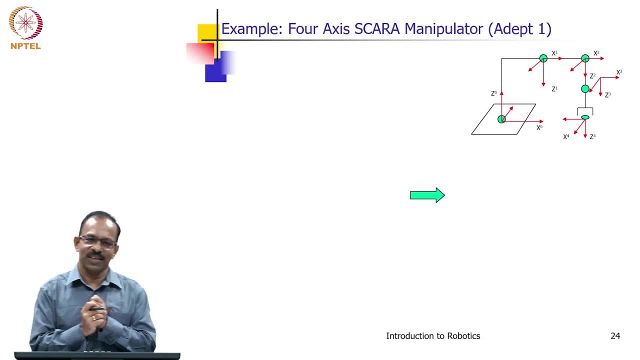 axis. So just to ensure that you are thorough with this process, so I am just showing one more example. So again, you will be getting Px like this: if you do a forward kinematics, you will be getting Px as L1, C1.. 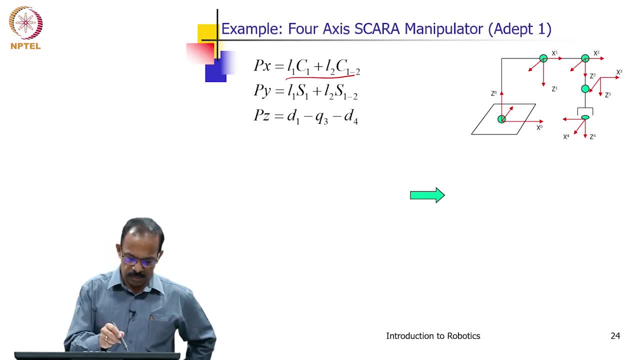 So Px is L1 plus L2, C1 minus 2, then Py is L1, S1 plus L2, S1 minus 2 and Pz is D1 minus Q3 minus D4. So in this case it is a linear joint. so you have one linear joint. that is why it is known. 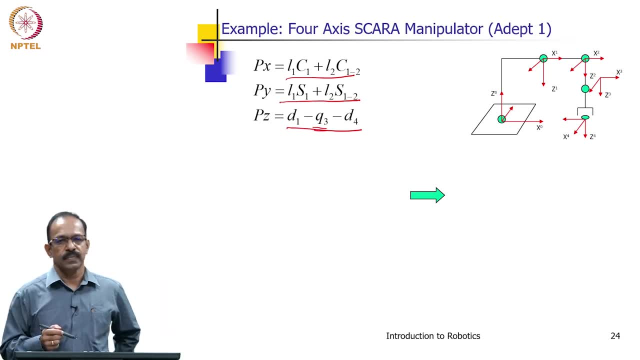 as Q3. it is the variable joint 3- sorry, the last one is basically a sorry. the third one is a prismatic joint. that is why Q3 is a variable. So this is a linear joint. So you have one linear joint. that is why it is known as Q3.. 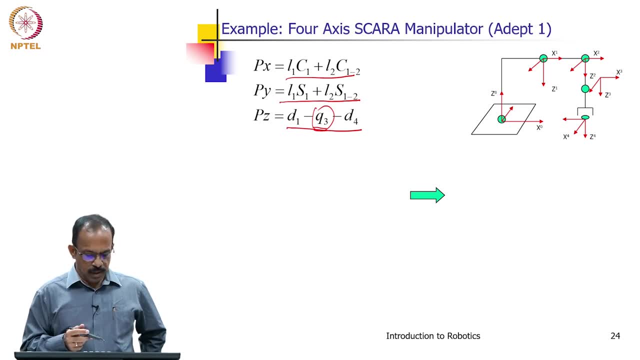 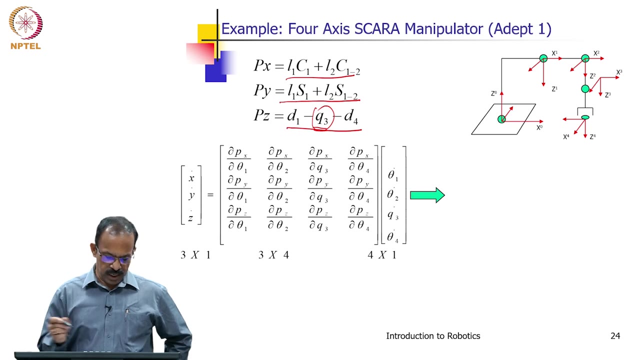 And D4 is a constant. Again the same principle. you apply the take the partial derivative with respect to theta 1, theta 2 and Q3 and theta 4.. So here you have Px with respect to theta 1, theta 2, theta 3- sorry, Q3 and theta 4: same. 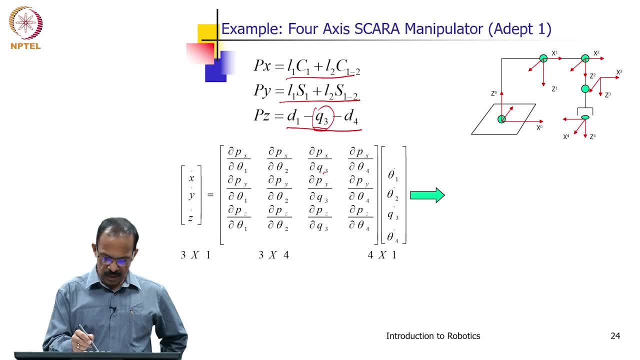 Py, Pz also. So these are the joint velocities: theta 2, theta 3.. So this is a linear joint, So this is a linear joint, So this is a linear joint. So theta 1, theta 2, Q3 and theta 4, and if you do this partial derivative, you will be. 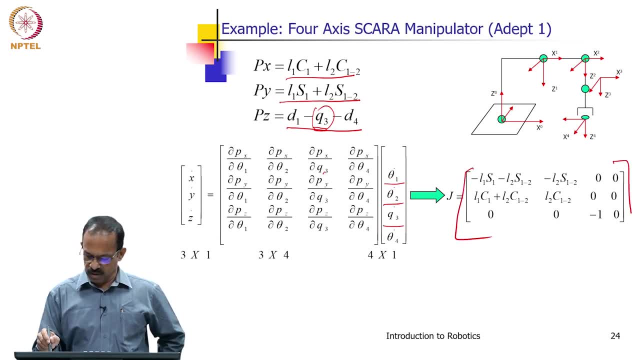 getting it as this. So Jacobian will be this matrix: minus l1, S1 minus l2, S1 minus 2, minus l2, S1 minus 2, like that. So you will be able to get the linear part of the Jacobian by taking the partial derivative. 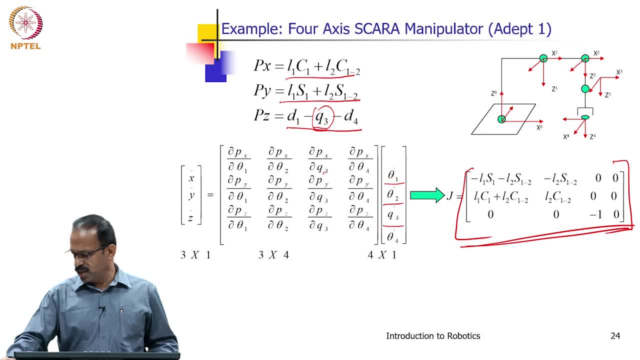 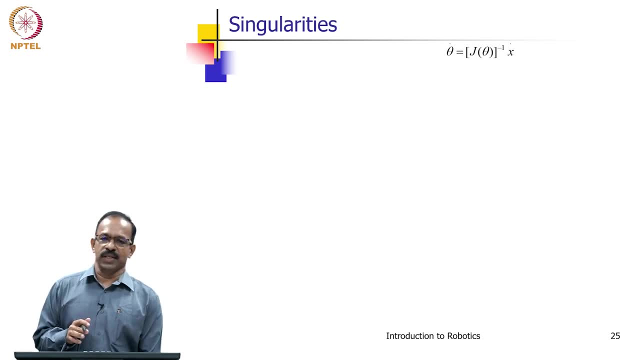 like this. I hope you understood this method. So let us briefly talk about the issues with Jacobian when we try to do the inverse. So, as I mentioned, you can do the theta dot by taking the Jacobian inverse. If you know x dot, you will be able to calculate theta dot. 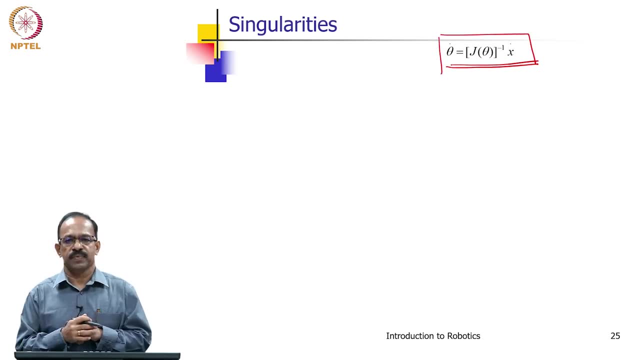 by taking the inverse of the Jacobian J inverse. But many cases you will be having difficulty in the in calculating the J inverse because J is a function of theta, So the Jacobian is a function of theta, as you saw in the previous cases. you can see this is. 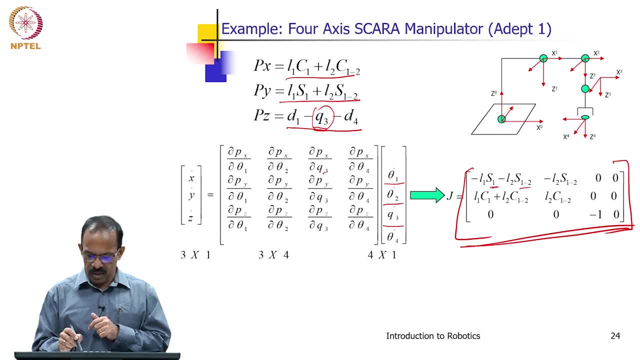 a function of theta. As theta value changes, the Jacobian matrix also changes. So for any different positions of the tool tip you have different matrix. the elements of matrix changes, So your Jacobian matrix also changes. So it is not fixed for a manipulator. 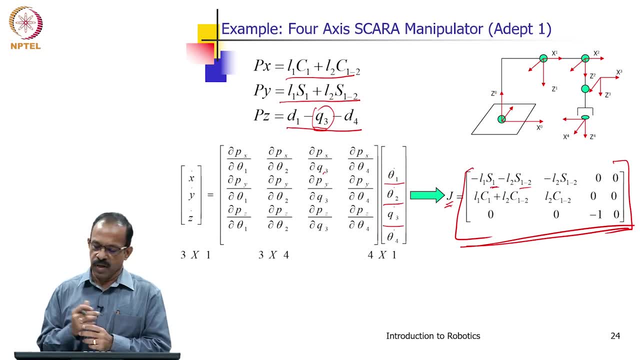 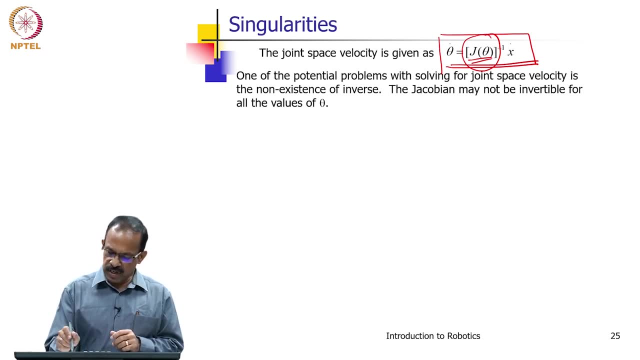 As the position changes, your J also varies And there may be some position in the workspace that this J become non invertible. That is when that is moving or when the theta value changes. there may be a situation where the Jacobian may not be invertible. for. 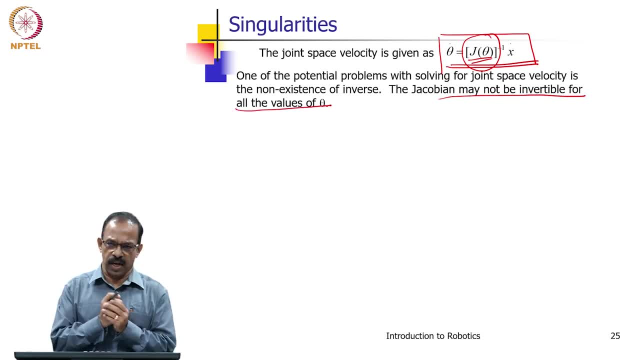 all ignore orflater. But that means the solution of this θ value changes, So it the values of theta, Assuming that J is a square matrix for the time being. in that case, also, when the matrix, the manipulator, is moving in the workspace, then you will see that at. 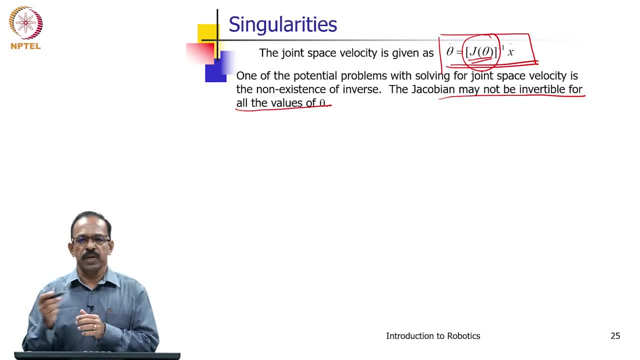 some. for some values of theta the Jacobian may not be invertible. That is because the Jacobian loses its rank. So if it is a 6 by 6 matrix, then the rank of the Jacobian will actually come down to 5 at some point. then you would not be able to invert it. So 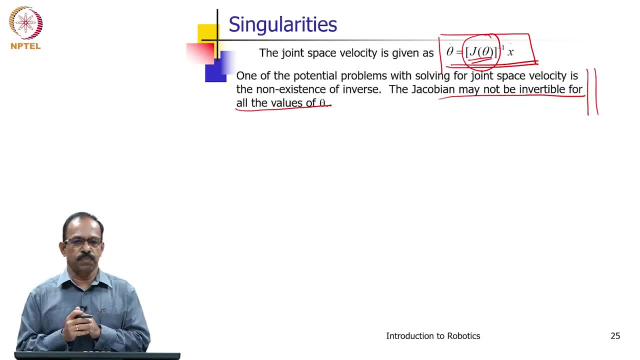 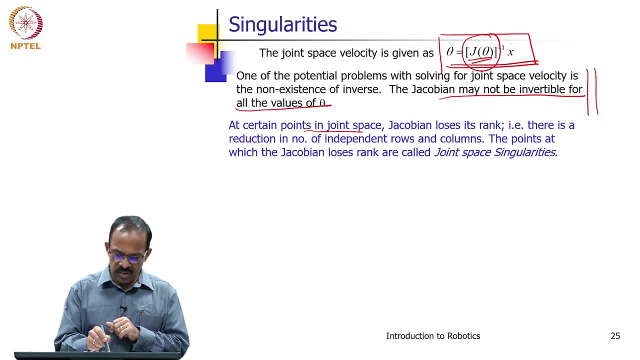 that kind of situations will be common in manipulator workspace and that kind of situations are known as singularity. So at certain points in joint space Jacobian loses its rank. For some values of theta the Jacobian loses its rank and there is a reduction in number of. 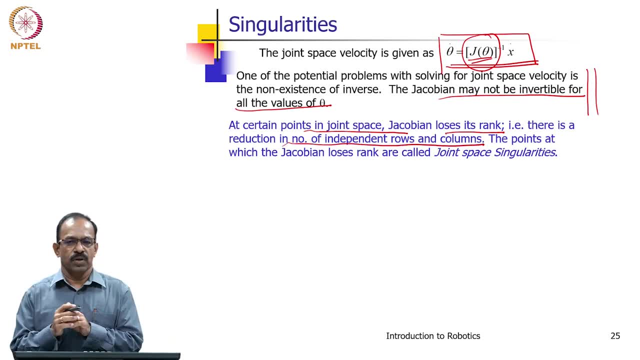 independent rows and columns in the Jacobian. So initially it was a 6 by 6 matrix, but then after some time It actually become. matrix is still 6 by 6, but the independent rows or columns reduced. reduces because of the position of theta and it loses rank. it becomes 5.. That situation- 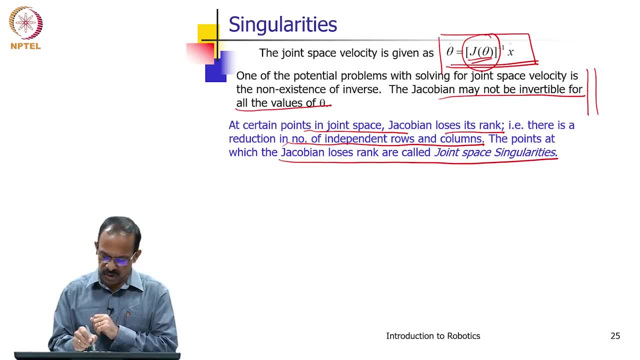 then you- such situations are called as joint space singularities- and you would not be able to invert the Jacobian at that point. And when you are not able to invert, you would not be able to find a theta dot Because you have an x dot, and at that point you will. 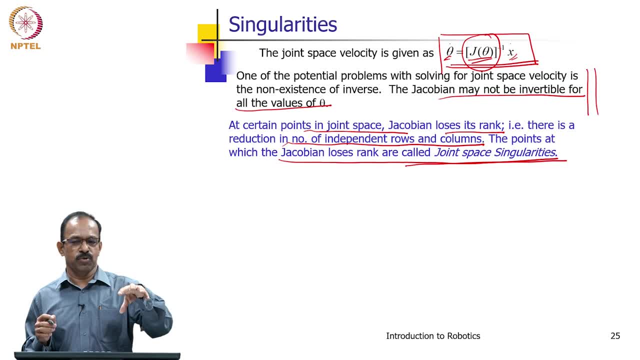 find that particular configuration of the manipulator, that particular joint positions. you find that J inverse is not existing and therefore you find it theta dot cannot be calculated, or you, for any values of x dot, you would not be able to find a theta dot. 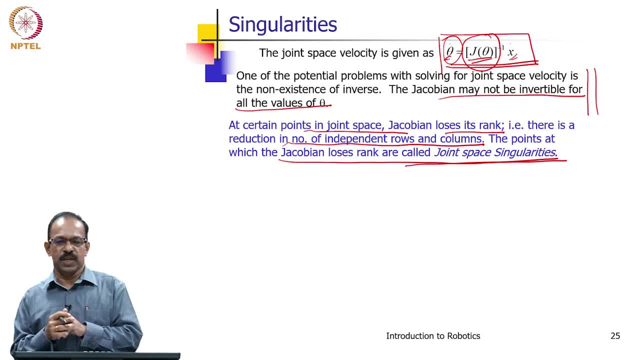 For any theta dots, you would not be able to get an x dot. So if you look at from the other point, you want to move the joint, you want to command the joint at very high velocity, but still you are not able to get the desired x dots. So this situation is known as the 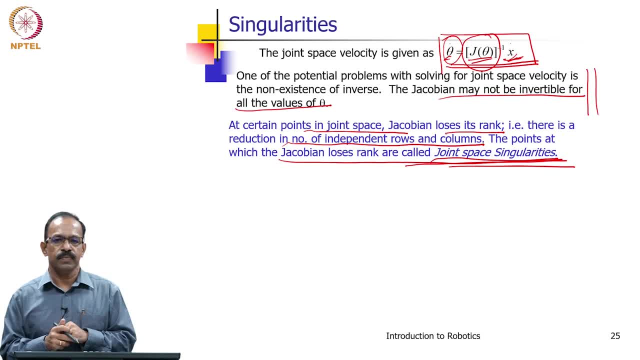 joint space singularities, And this is common because the Jacobian, since it is a function of theta, as the theta takes a particular set of value, then for that particular set of value we will see that this relationship is not possible to be evaluated, or any value. 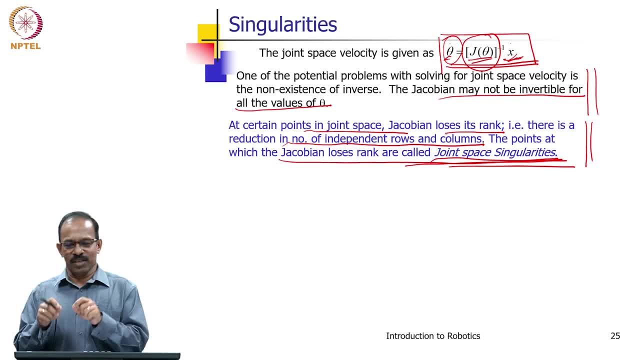 of theta dot, you would not be able to get an x dot. or to get an x dot, decide x dot. the theta dot should be infinite. That is the way how you can look at it. If you want to have an x dot, then you need to have an infinite velocity at the joint to get this. 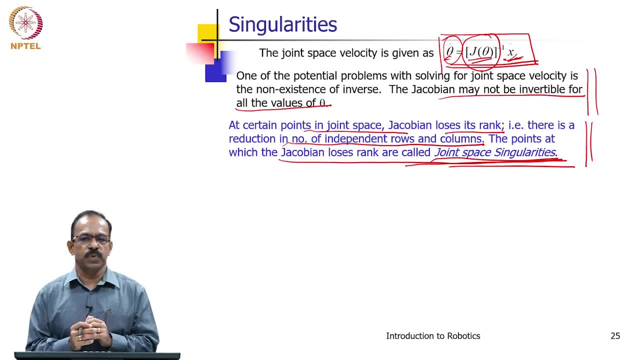 x dot. Such situations are known as joint space singularities, or that position of that manipulator is known as singular point or a singular point in the workspace. It can be multiple points, need not be a single point. it can be multiple points or as it reaches. 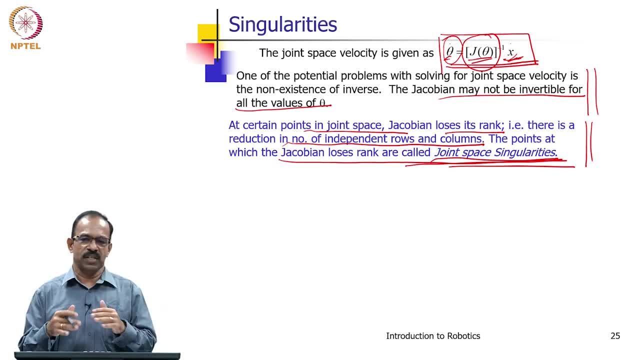 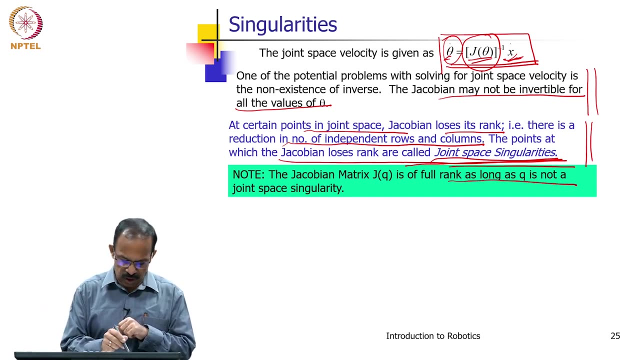 the that point, You will find that the manipulator, the Jacobian, loses its rank. So this situation is the joint space singularity. So the Jacobian matrix JQ is of full rank as long as Q is not a joint space singularity. So the JQ will be of full rank as long as the Q is not. 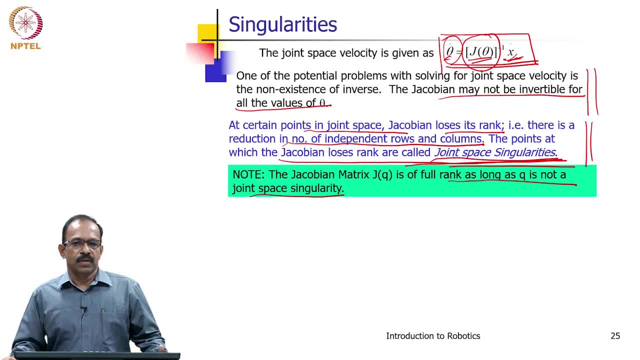 a joint space singularity. So when it is a singular at the joint space, that singularity, Then the JQ loses its rank And this can actually be measured by something called a dexterity measure. So how close the manipulator is to a singular point can be measured by the 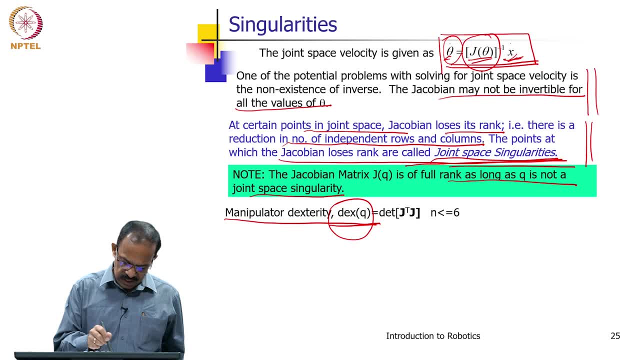 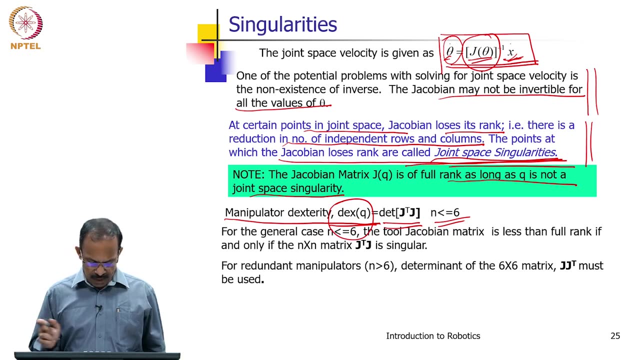 term dexterity, So we would measure this as dexterity. we define dexterity as the determinant of J transpose, J or J. J transpose, depending on the value of n- is less than or equal to 6 or more than 6.. So this is used to get the dexterity measure. If it is n greater than 6, then we use J- J. 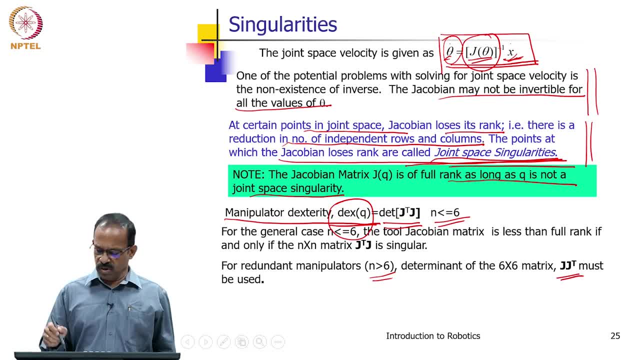 transpose. So either J transpose J or J J transpose, we find out the determinant of J, J transpose, and that is known as that is. that will give you the dexterity of the manipulator. And for the general case, the tool Jacobian matrix is less than full rank. if, then only 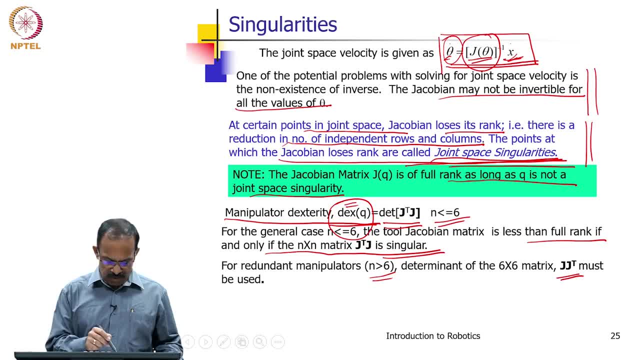 n by n. matrix J is singular And for redundant manipulators, determinant of 6 by 6 matrix must be used. This is for when the n is less than 6 or more than 6, you need to use J transpose J or J J transpose. Now a manipulator is a joint space. singularity if, and only if, dexterity. 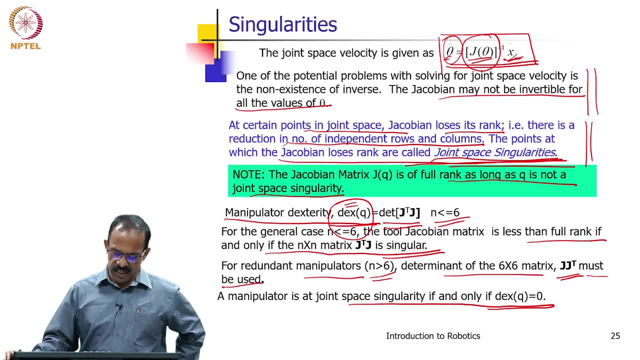 is 0. So when the dexterity is 0, that is, the determinant is 0 for J transpose, J or J J transpose, then we call this as the singularity, or that space singularity, dexterity will be 0. So when manipulator is starting from one point which is not a singular point or the 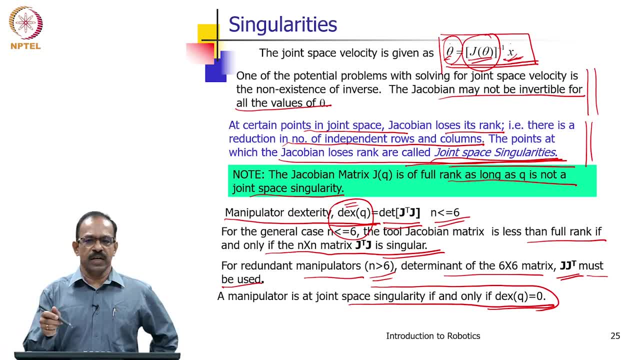 dexterity is very high, then this value will be having a very high value. Then, as it moves towards the singular point, you will be getting it as 0. So as it moves to the singularity singular point, it will start coming down very small values and then finally, at the 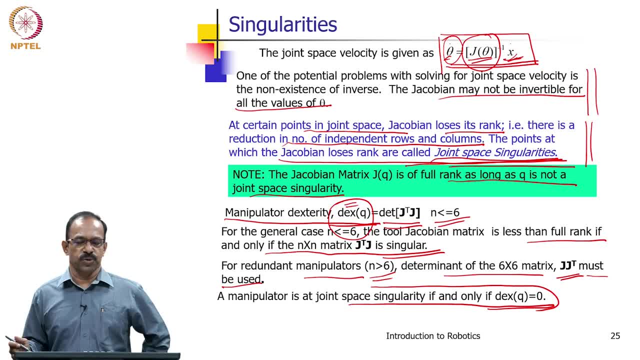 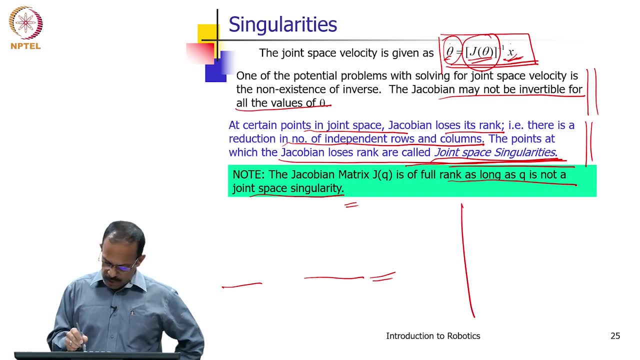 singular point, you will be getting a dexterity value as 0. So this is actually a measure of singular space. I mean this dexterity, that is, if you have a manipulator workspace. so if you have a manipulator workspace like this, then there may be a singular point somewhere. 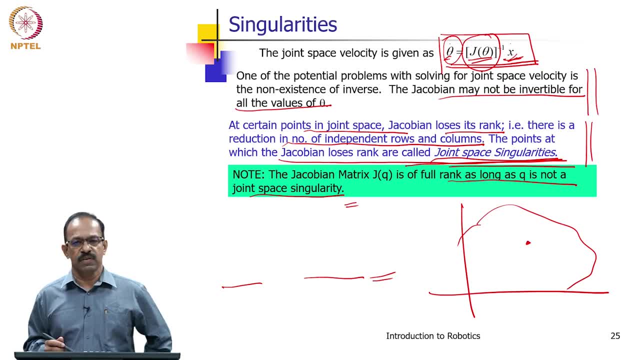 here. So this is a singular point here and at this point the dexterity will be 0. And other places you will see that as it moves here, the dexterity will start coming down to 0. So it may be having some value of dexterity here, but as it moves towards this, you will see that it. 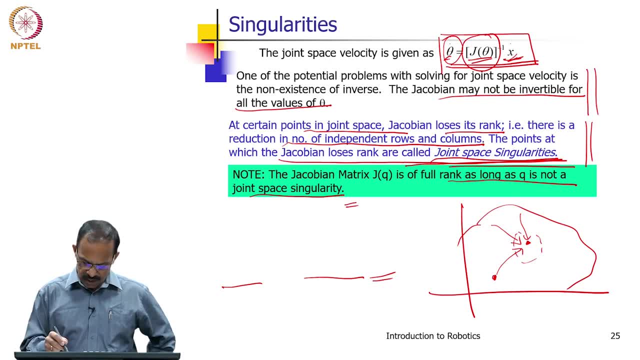 actually comes down to 0. So neighborhood of this will be having very small value of dexterity and again you will find difficulty in moving the manipulator in this area, This whole area, you will find difficulty because the dexterity has come down and therefore 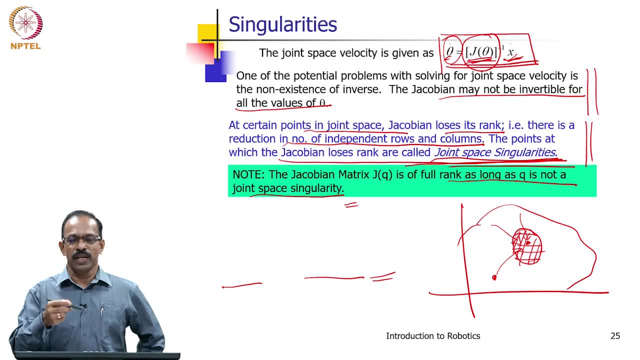 this will have difficulty in getting the inverse, So the theta dot will keep on increasing as it as it goes close to this area. So for getting a different constant velocity: if you want this to move with the constant velocity along this path, then you find that 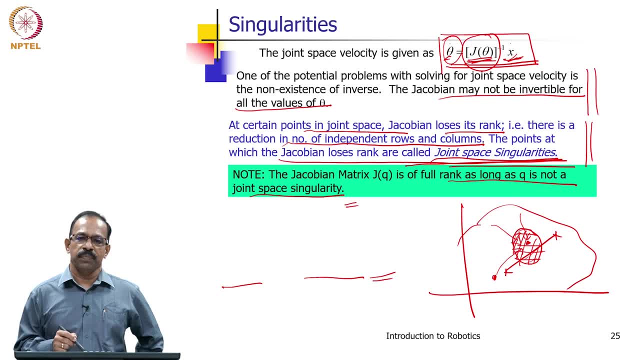 as it passes here, this area, you will be having difficulty in getting the desired velocity. And if it has to pass through this, then you will say somewhere: here it will be getting the desired velocity. So that is the way how the dexterity measure is used to find. 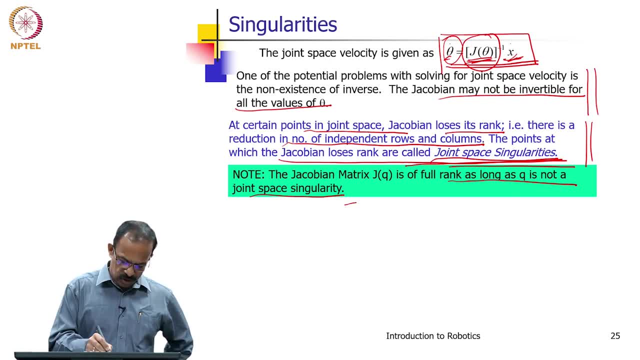 out the dexterous workspace of the manipulator. So every manipulator will be having a dexterous workspace where the dexterity is very high And other spaces where actually dexterity is low. we will try to avoid going towards to going that space. So the manipulator when 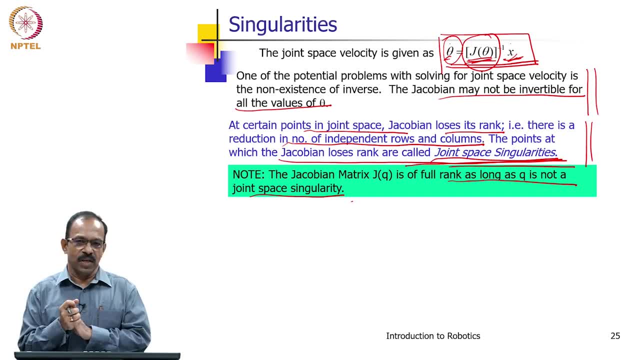 you design the manipulator. we look at the dexterous workspace and we ensure that most of the our operations, So this will be done within the dexterous workspace and we try to avoid the other workspace for normal operations. And if you want to move to some other point, we also try to avoid 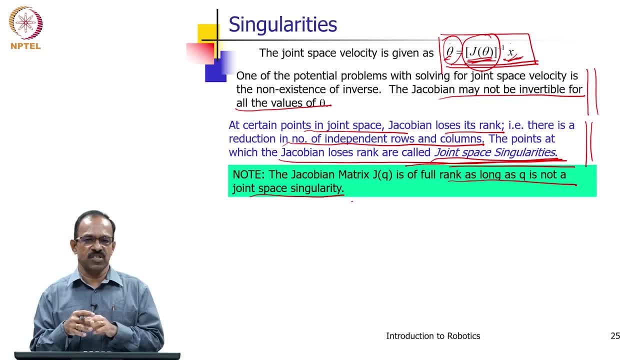 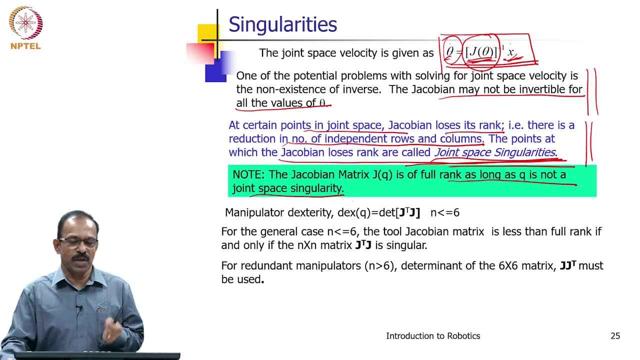 the dexterous space and then move, or we will plan a path in such a way that the singular space is avoided and then the robot is moving to the target. That is the importance of knowing the dexterity of the manipulator And then, as j is a function of theta, you will be able 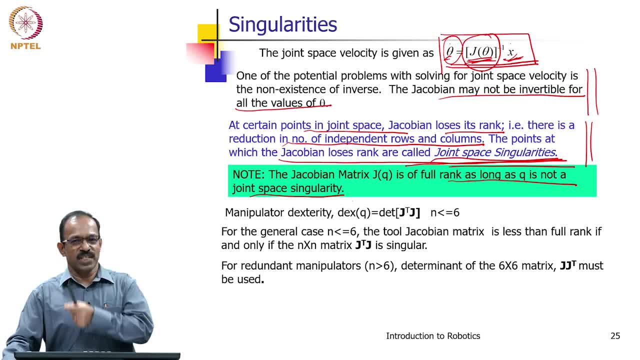 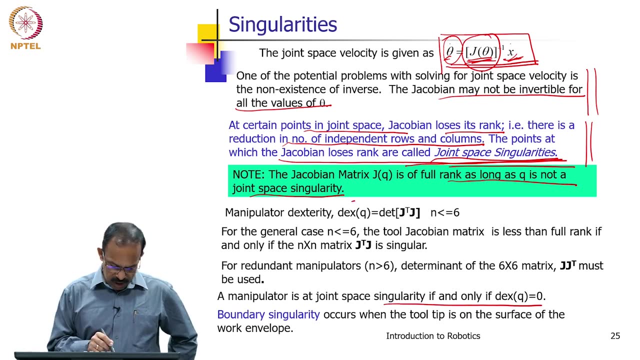 to find out the dexterity of- I mean dexterity at every point in the workspace, and you can make a plot of the dexterous workspace. So there is the singularity when, then, there is something called boundary singularity. boundary singularity occurs when the tool tip is on the surface of the work envelope. 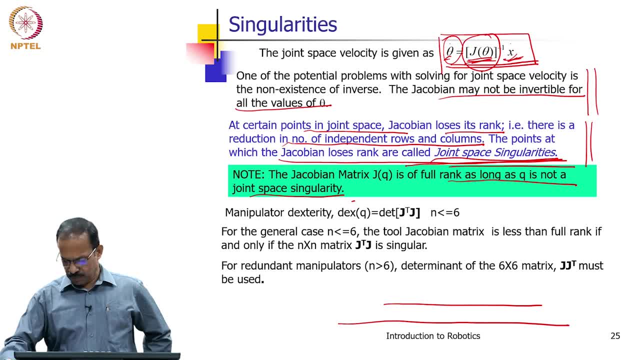 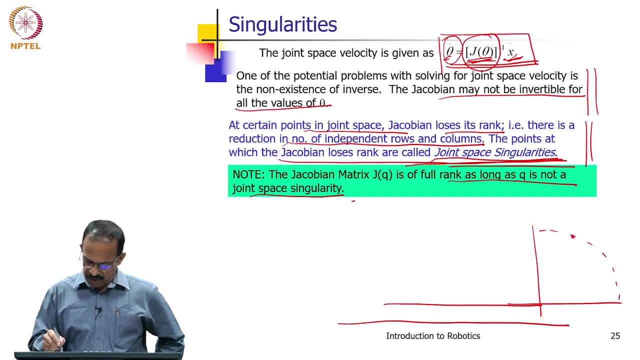 that is, when you have a workspace. When you have a workspace like this, Okay, And the tooltip has already reached here. the tooltip has already reached this position, then we call this as a ok. this will not be the right representation, so the tooltip 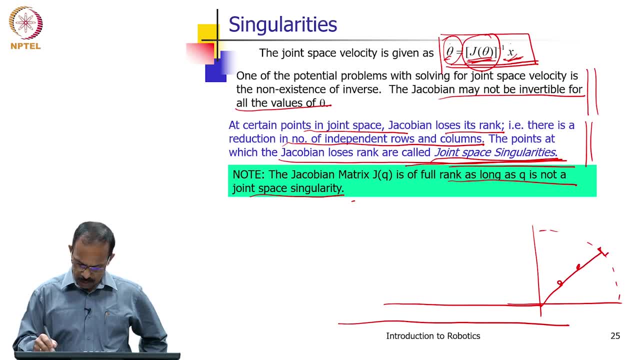 has already reached this point. Now, this is also a kind of singularity, because if you want to move it in this direction, you will not be able to move. if you want to give a velocity in this direction, then you will not be able to move. you have actually reached the maximum that you can reach, and 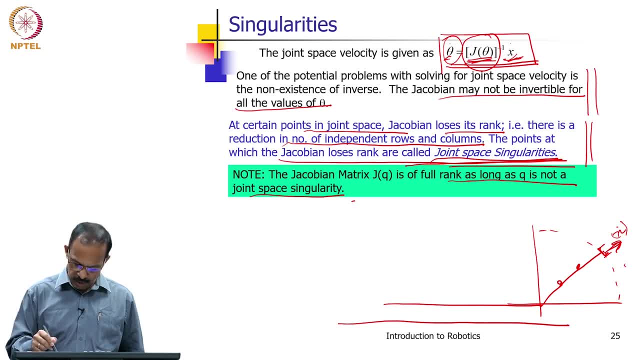 then again you have a velocity in this direction you will not be able to give, but you can actually move in this other directions, you can move in this direction or this direction, but you cannot move in this direction. So that is a kind of singularity, and that we call it as the boundary singularity of 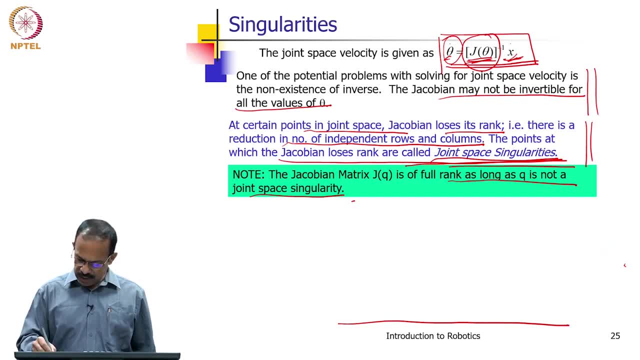 the manipulator, But you can have it in inside. that is the interior singularity, Ok. And when it is at the boundary, we call it as boundary singularity, And boundary singularity exists for all manipulators. you cannot have velocities in particular direction. 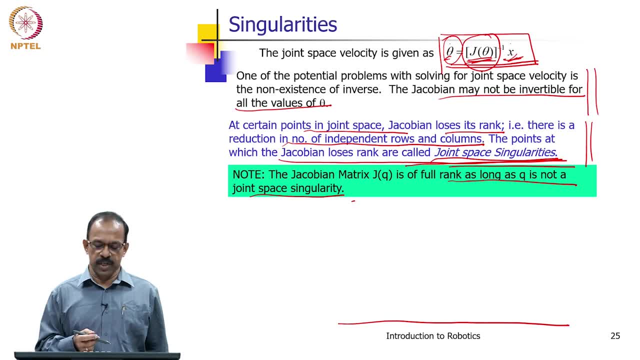 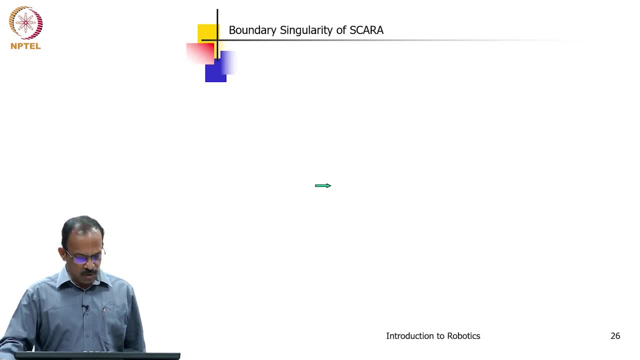 when the manipulator has already reached the boundary. So that is boundary singularity and the other one is the interior singularity. Just to tell you what is to explain you how the boundary singularity is calculated. so look at this manipulator for the manipulator, where you have a Jacobian manipulator. 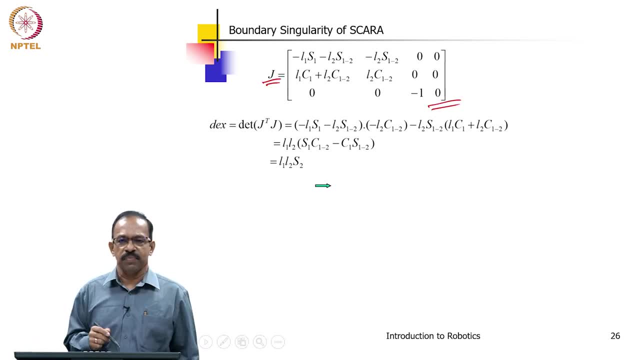 So we saw this Jacobian for the manipulator. now, if you have a Jacobian like this, we can find out what is the boundary singularity of this manipulator. What we need to do is to find out the dexterity and then see when the dexterity will be 0.. 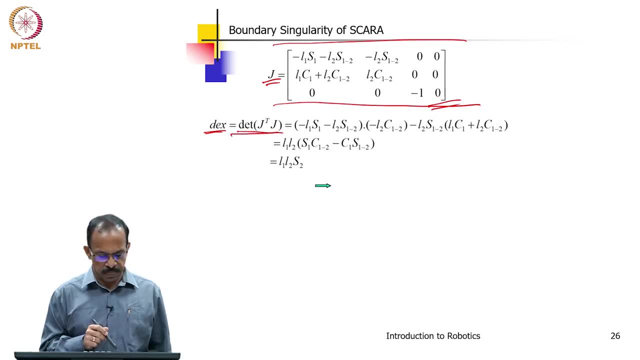 So we can identify this dexterity as like this: determine J, transpose J and then find out: this is the dexterity in terms of the joint angles. Ok, So we will see that L1, L2, S2 is the dexterity, and this will be 0 when S2 is 0. 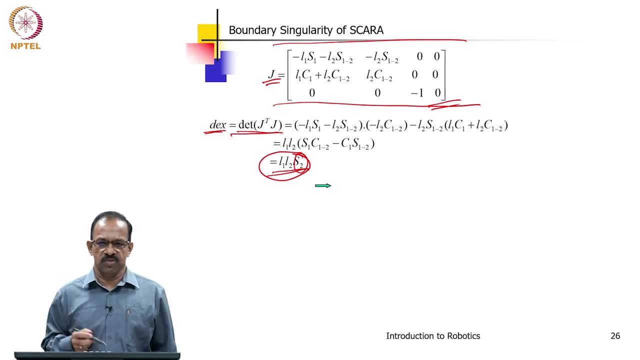 So when your sin theta 2 is 0, you will be getting dexterity as 0 and that will be the boundary singularity. You can see that when theta 2 is 0 or pi, the manipulator will be singular. So this is the case for the Scara robots. so you can see that when it is fully extended, 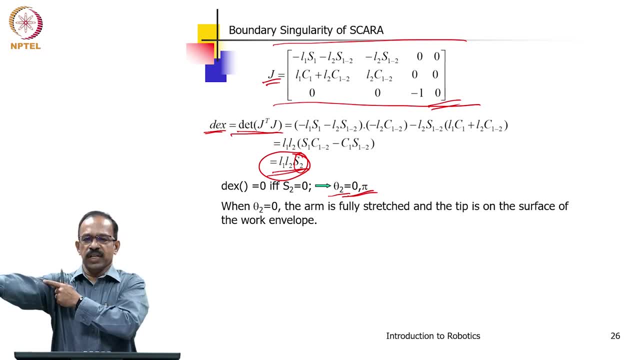 then it is at the boundary And theta 2 is 0, it is at the boundary, so it is a singular configuration. Similarly, when it is fully closed, then it is, theta 2 is pi. again it is at the boundary. 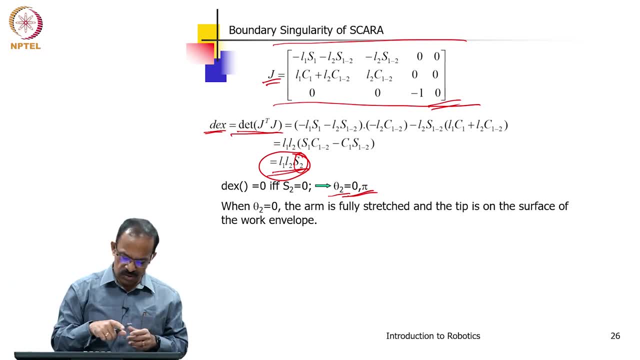 so again, boundary singularity. So you will see that this theta 2 is equal to 0 over pi is a boundary singularity for the manipulator. So this is how we get the boundary singularity of any manipulator we can actually find out. 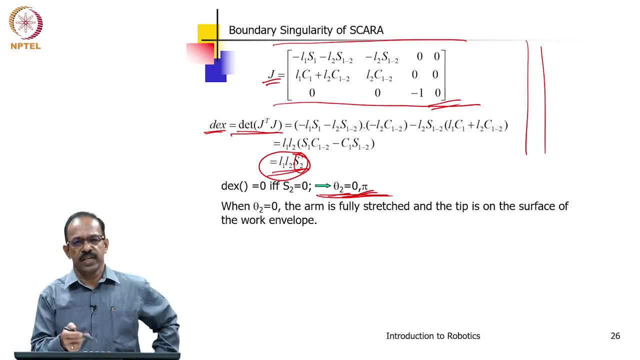 the manipulator boundary singularities by finding out the dexterity of the manipulator. Ok, So finding out the dexterity when it actually will become 0, then you will be able to find out the boundary singularities. So, whenever theta 2 is 0, it is actually a 0 over pi, then it will be a boundary singularity. 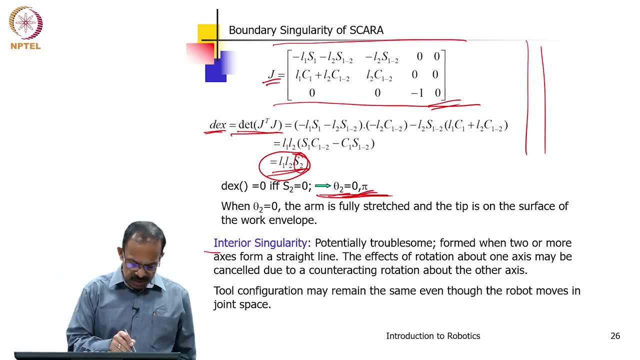 That is about the boundary singularity And the interior singularity. as I mentioned, it can actually happen. it is a very troublesome. So boundary singularity is not a problem, but interior singularity is an issue. It is formed when two or more axes form a circle. 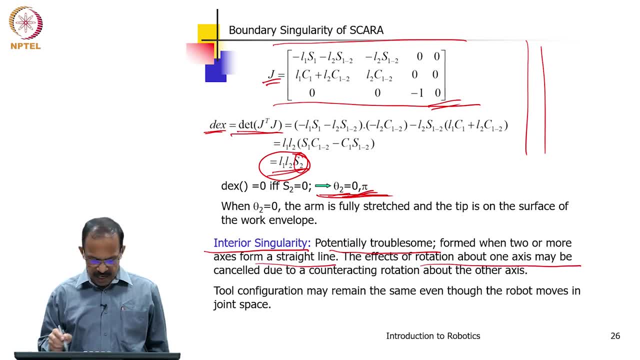 Ok. When two or more axes form a straight line, the effects of rotation about one axis may be cancelled due to counteracting rotation about the other axis. So this kind of singularities can happen when you have one rotation happening but other rotations of the joints actually counteracts. 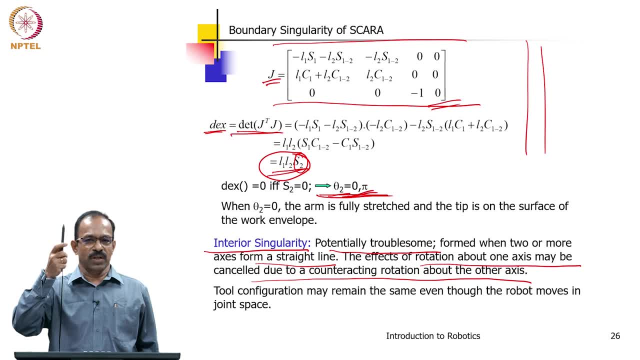 And therefore, even if the joints are moving, your tool tip is not moving. Ok, So you have a joint velocity, but you do not see any movement at the tip, or the Cartesian velocity becomes 0 when your joint velocity is still acting. that kind of situations also. 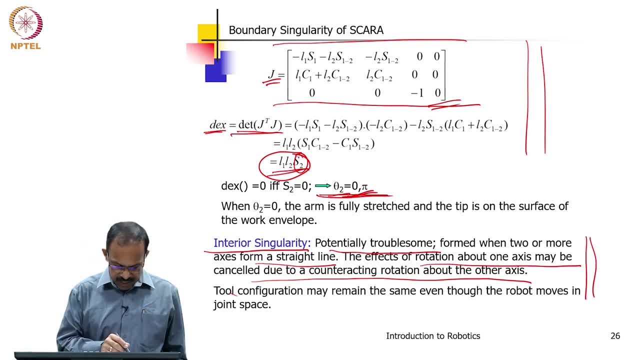 known as the interior singularities. So the tool configuration may remain same, even though the robot moves in joint space. So the joint space, the robot is actually moving, but the tool configuration space- no movement is taking place. So that kind of situations are known as interior singularity. 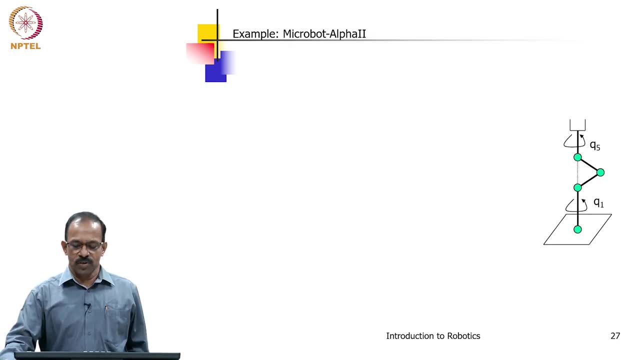 So let us take this example for the micro robot alpha: Ok, And then see how the interior singularity- Ok, And then see how the interior singularity happens in this case. So we can see this configuration of the robot. So the robot has actually reached a configuration like this. 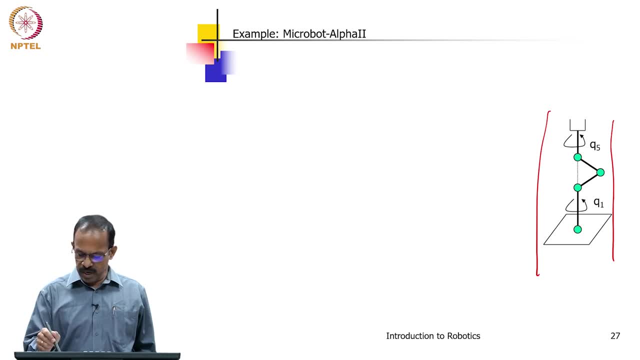 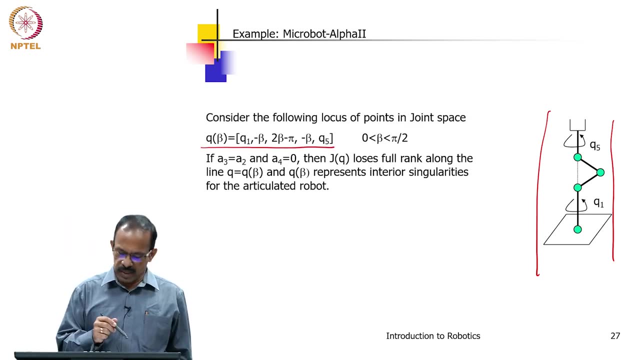 So now this, the robot joints are actually positioned like this And you will see that this Qb, that is, the joint angles, are like this: Q1 minus beta, 2 beta minus pi minus beta and Q phi. So this is Q1 and this is Q phi. 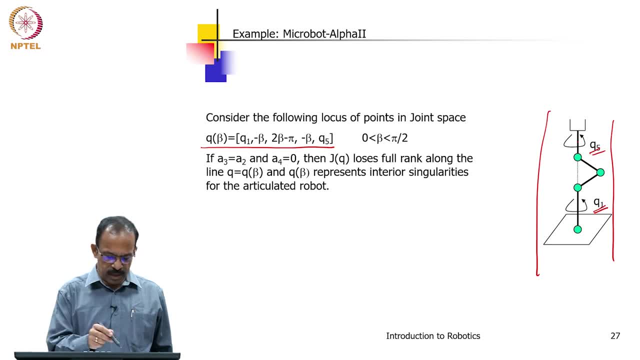 So this is Q1 and Q phi. Ok, So these joints are like: minus beta, 2, beta minus pi and minus beta. So other two, three joint angles are like this: where beta is less than pi by 2, between: 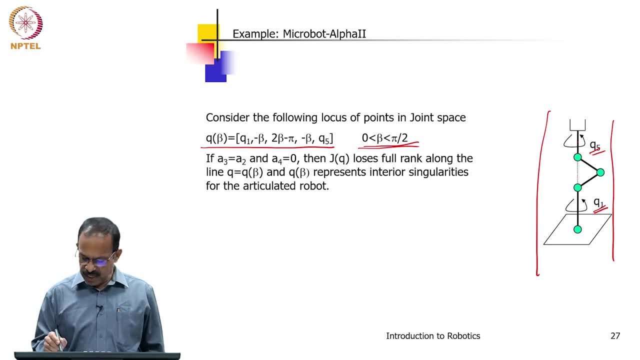 0 and pi by 2.. And then this situation: you will see that even if Q1,, Q1 is having making an angle and then Q phi is making a opposite rotation, then this will actually remain same. There will not be any change in the position and orientation of the end effector, even. 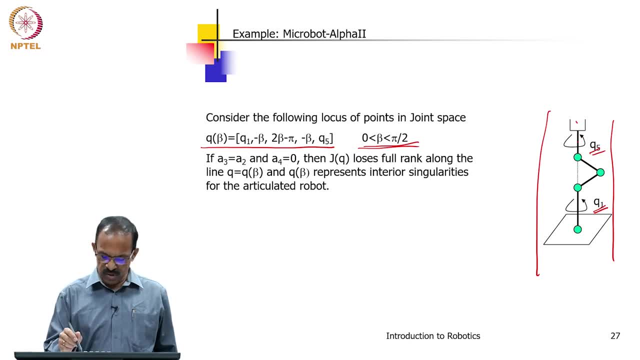 if Q1 and Q phi are making minus beta, So that kind of a situation is known as interior singularity- Provider a3 is equal to a2 and a4 is equal to 0. Then Jq loses full rank along the line q beta, and q beta represents the interior singularities. 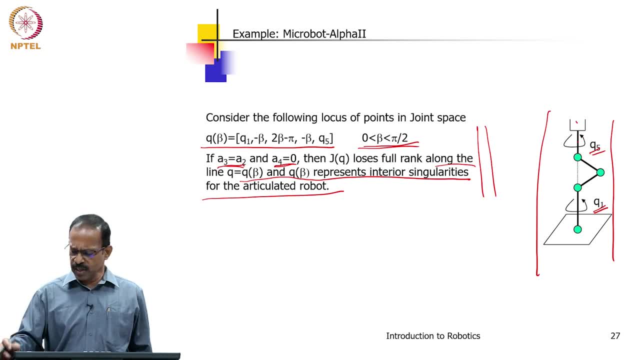 of the articulated robots. So these kinds of situations will arise when it actually aligns in a particular way, and I mean the joint angles and the parameters are in such aligned in such a way that you have this kind of situation where the tool line is going to be constant. 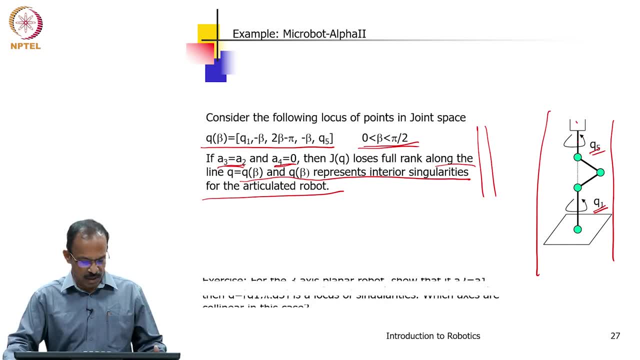 Ok, tip is not moving, even if the joints are moving. So that is basically known as the interior singularity. So this particular robot has got an interior singularity like this. So this is an exercise for you, for the three axis planar robots show that if a2 is equal, 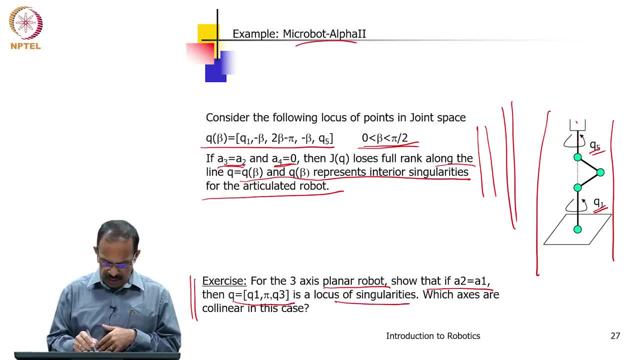 to a1 and then q1 by. q3 is a locus of singularities. which axis are collinear in this case? So let us try to see how this interior singularity happens and which are the axis that are collinear, in this case, The planar robots. and a2 is equal to a1, so you will be able to see the 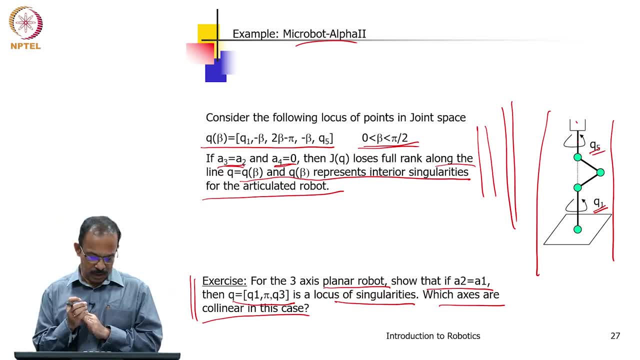 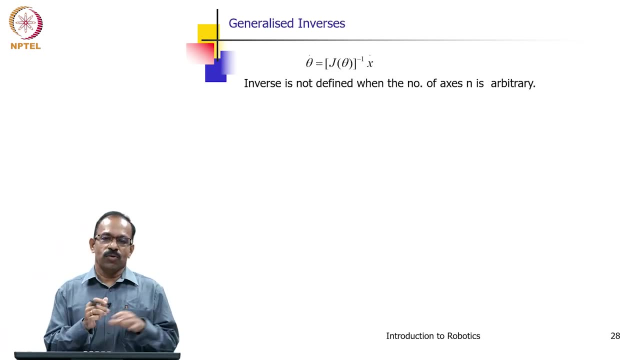 situation why it is getting locus of singularities, So that is, the singularities in the manipulator. Now, So we mentioned that whenever this j is not invertible because of the position of joint or the joint space, values or joint variables are in such a way that the matrix loses its 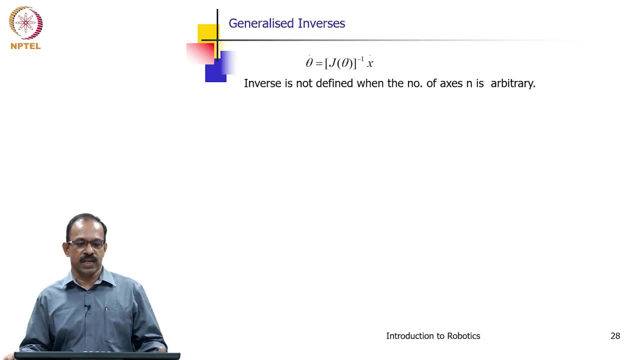 rank. So that is one situation where actually you can get singularity. Another problem with this inverse j inverse is that when it is non-square matrix, you will not be able to get the inverse. So when it is a 6 by 5 matrix, you will not be able to get the inverse of j. 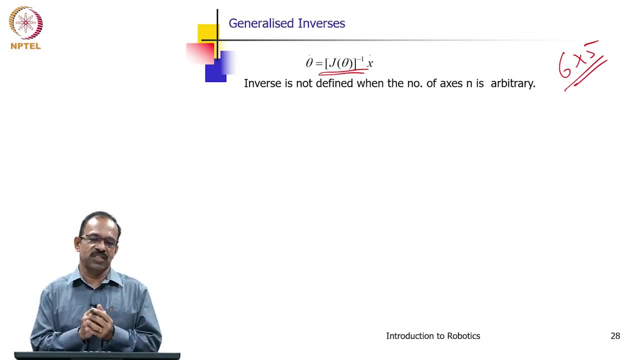 So how do we actually solve this? So one is that the j loses its rank, you do not have any inverse. and there the other one is: j is not a square matrix, you do not get a inverse. So that is the situation where you encounter in the manipulators which are having degrees. 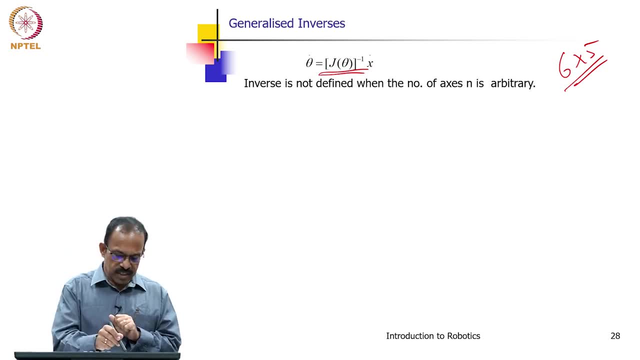 of freedom other than 6.. So in this case what we need to do is to get an inverse to some other means, and that is known as the generalized inverse. So a non-square matrix can be inverted and we can use something called a generalized. 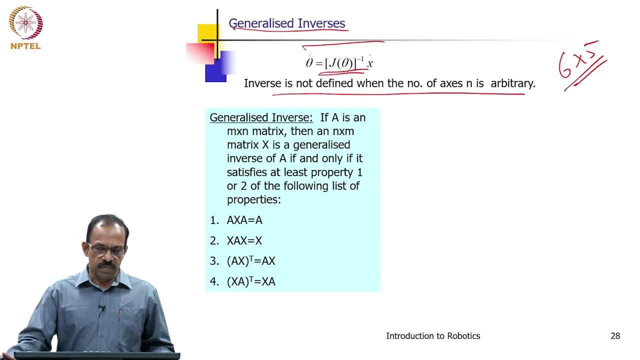 inverse in this case. So this is defined as a generalized inverse, is defined as if A is an m by n matrix. so if A is an m by n matrix, Then m matrix X is a generalized inverse of A if and only if it satisfy at least property. 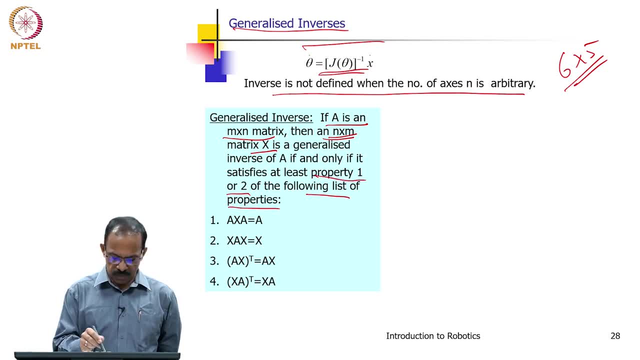 1 or 2 of the following list of properties. So if A is an m by n matrix, then we can have a X as an n by m matrix, as the inverse of A, provided it satisfies at least 1 or 2 of this property, that is, A X, A is equal to A and X A. X is equal to X. So if we can actually 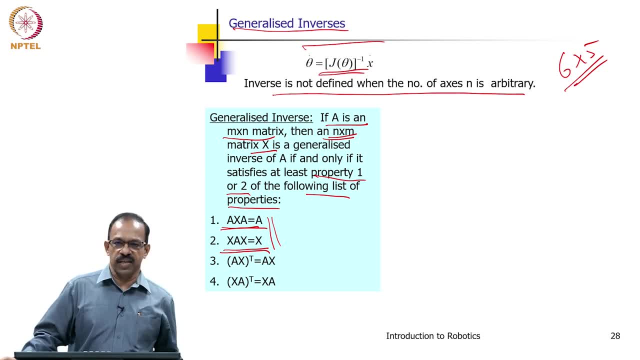 have a matrix like that- X is like that, A X, A is A and X A, X is X, then we say X is a generalized inverse of A If it satisfies property 1 or 2 of the this, that is, this 1 or 2, it satisfy A X, A or X A X, then we call it as a generalized inverse. 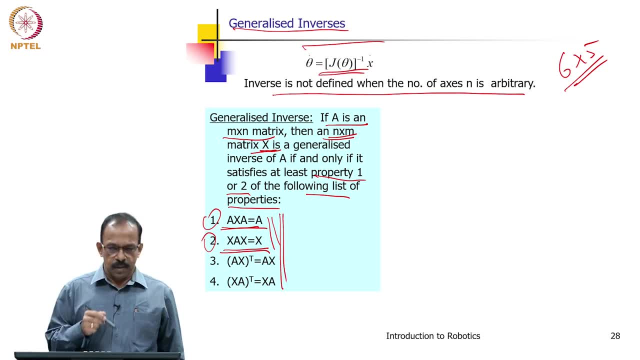 And therefore, once we have that X as a generalized inverse- I mean we can have X as a generalized inverse- then we will be able to get the J. J is m by n. we can find a m by n matrix which satisfy this condition, then we will get that as the inverse. So that is known as the generalized. 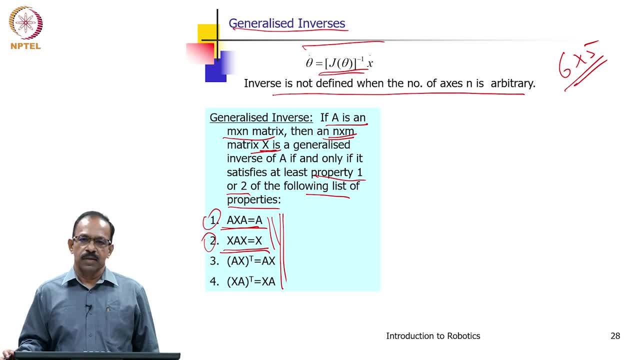 inverse of a non-square matrix. Now a very commonly used generalized inverse is known as Moore's law Moore Penrose inverse. Moore Penrose inverse is known as a. it is very commonly used generalized inverse and sometimes it is known as a pseudo inverse or we call it as A plus. So A plus. 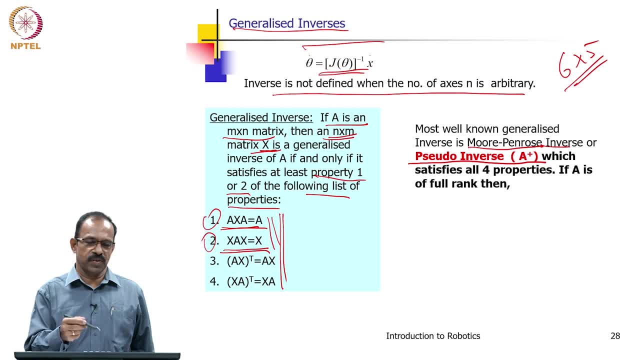 is known as a inverse of pseudo inverse of A. So instead of writing A inverse, we write it as A plus. it is a pseudo inverse and it satisfy all properties, if all properties listed here, So it actually satisfies all these properties. 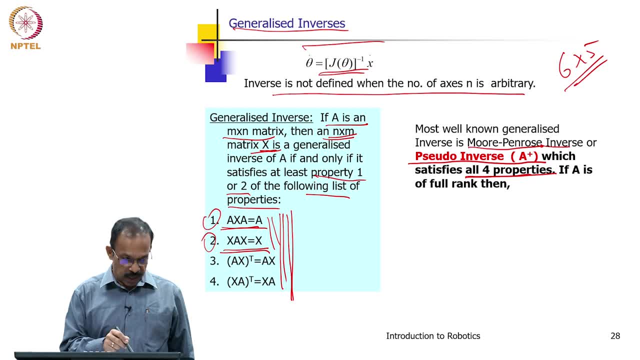 A A. So A X A is equal to A X, A, X is equal to X A, X transpose is equal to A X and X A transpose is equal to X A. So this Moore Penrose inverse, or the pseudo inverse, will satisfy all these. 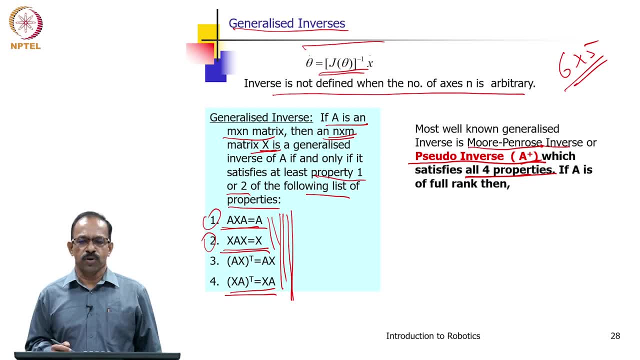 condition and therefore A plus will be an inverse of pseudo inverse of A, where A is a non-square matrix. And how do we get this If A is of full rank? so condition is that the A is of full rank. So if it is a rank 5 or rank 7, you will be able to get it as is a full rank then. 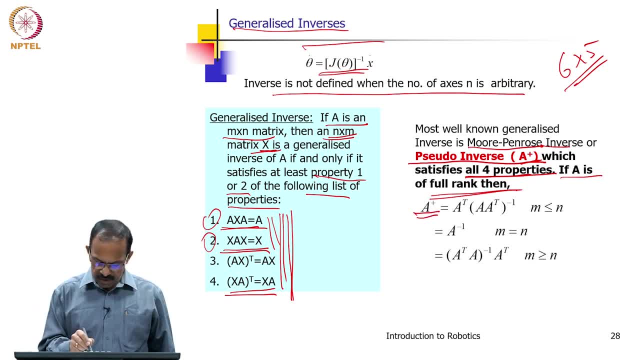 we will see A plus is given as A transpose A, A transpose inverse if m is less than or equal to n. Of course, if m is equal to n, then it is A inverse. only A plus will be A inverse. if it is a square matrix it will be the same, But if it is A inverse, then 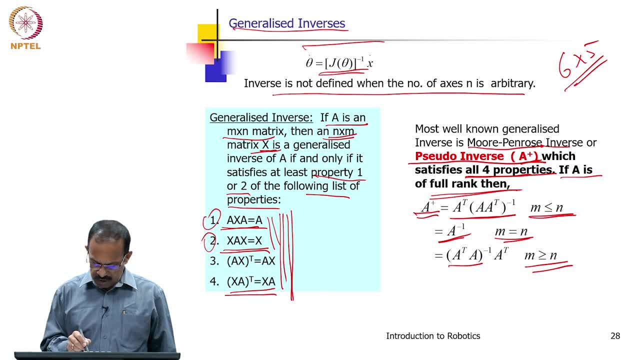 it is. if it is a square matrix, it will be a square matrix. So if m is greater than n, then A plus is A transpose, A inverse, then A transpose multiplied by A transpose. So this is the way how you get the pseudo inverse A plus. So pseudo inverse A plus can be obtained. 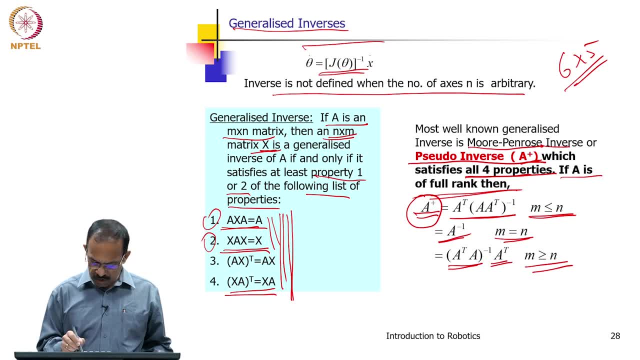 as either A transpose A, A transpose inverse, or A transpose- A inverse, A transpose, and m is greater than n. So now you can see. what we are doing is we are actually converting, converting this as a square matrix. So A- A transpose becomes a square matrix now, because 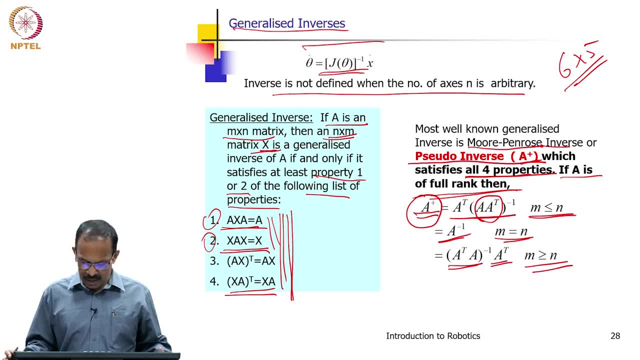 A is a non square matrix. So A- A transpose- becomes a square matrix and you find the inverse and multiply, pre, multiply with A transpose. or again here you convert that into a square matrix and get the inverse and then multiply with A transpose. So this way you will be. 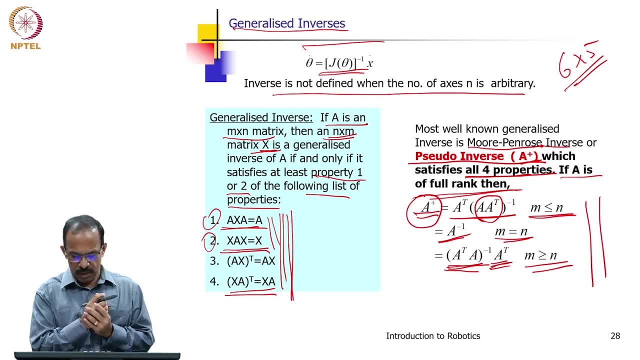 able to get the pseudo inverse of the manipulator, So that is known as A plus. I hope you got the point. So, even if the Jacobian is not a square matrix, we will be able to get the inverse using the Moore Penrose inverse method, or known as the pseudo inverse. 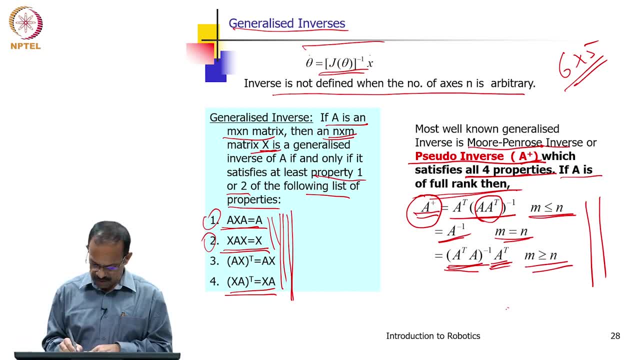 So you have J, then J transpose. So if your J is inverse is J plus will be A plus. So you have J transpose J, J transpose inverse if m is less than or equal to n. That is the way how you get the J plus. So you can always get use J plus and then solved for the. then. 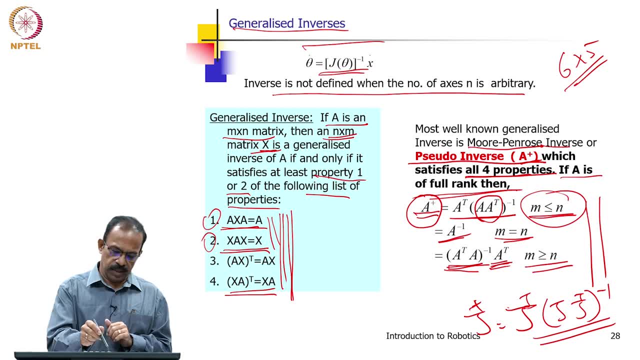 get the theta dot and get the values here. So non square matrix is not an issue. we will be able to solve it using the pseudo inverse, That is, the J transpose, j transpose and then get the theta dot and get the values here. 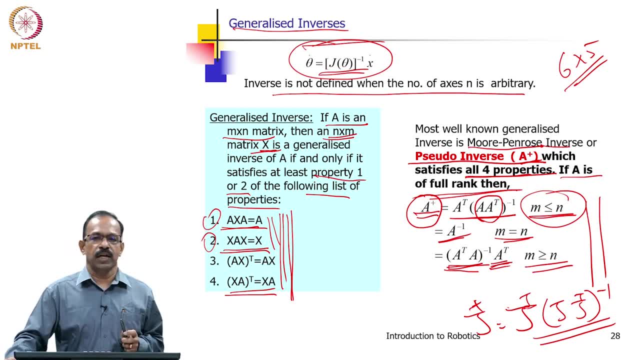 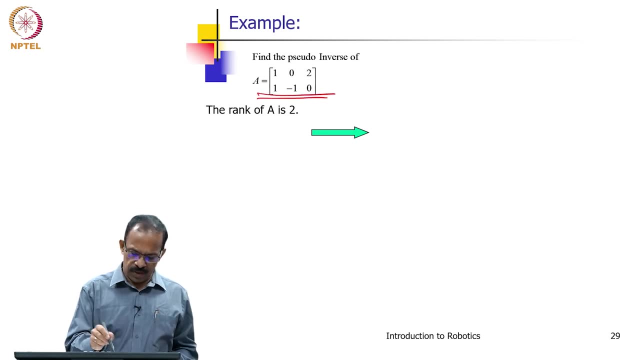 generalised inverse and how we use it for calculating the joint velocities, if we know the Cartesian velocity or the tool velocity, all right, So this is just an example for the pseudo inverse. Suppose you have a matrix A, it is 2 by 3 matrix. So m by n, m is 2 and n is 3 and the rank is A is 2, it is a full rank. 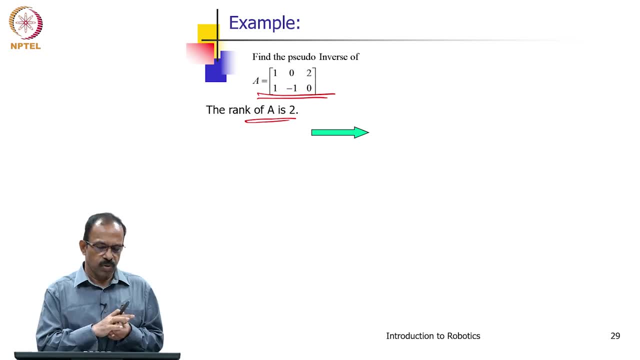 that is, the rank of the matrix is 2.. Now, if you want to apply the, get the pseudo inverse, we use the principle of that taking by converting this into a square matrix and then getting the inverse and multiplying with A transpose. So we will be getting it as A plus is A transpose. 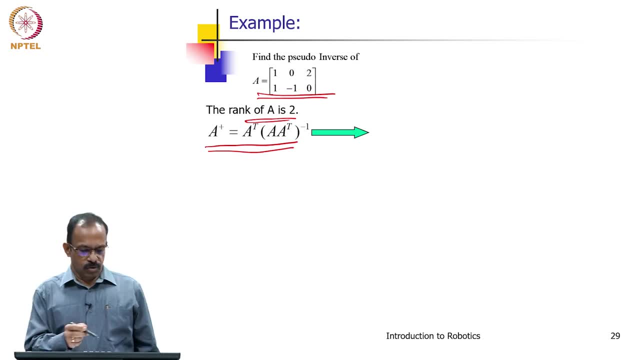 A, A transpose, inverse. So when you say A, A transpose, it is 2 by 3 multiplied by 3 by 2.. So it will be a 2 by 2 matrix. you get the inverse and multiply with A transpose. 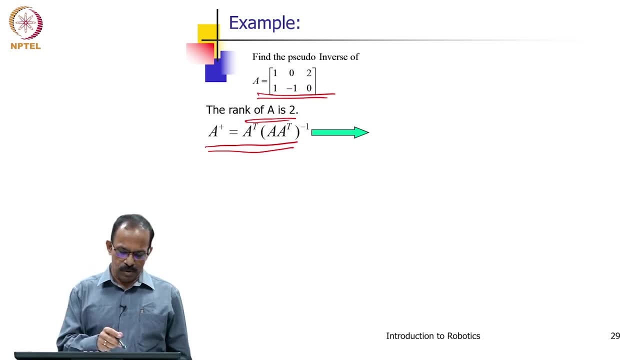 So you will be getting it as a 3 by 2 matrix, as the inverse. So A plus will be A will be a 2 by 3 and A plus will be a 3 by 2 matrix. So you will be getting this as the A plus. 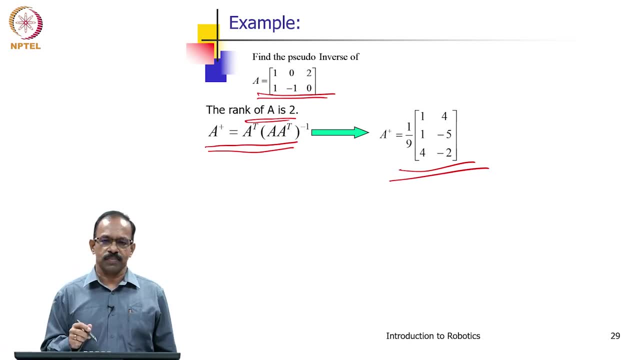 which is the inverse. So it is a 3 by 2 matrix and this is the pseudo inverse of A. So this is the way how we get the pseudo inverse and then, once you have, you can use it for getting the doing the calculation of A. 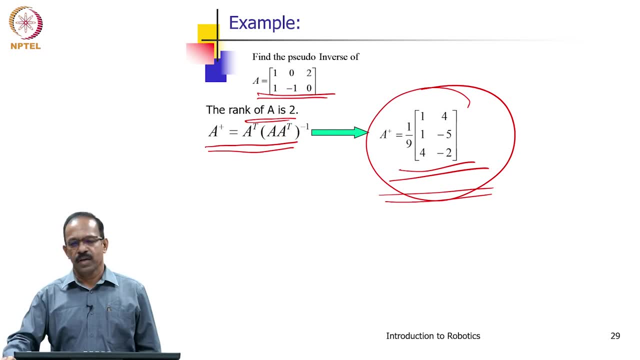 So there is one more question: what is the motion rate control in a joined velocity? We should beovy tech path and we should be doing the calculations of velocities in the case of Jacobian and getting the join velocities. What is the application of this particular 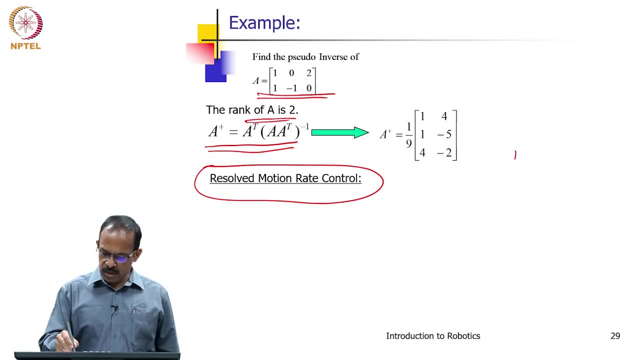 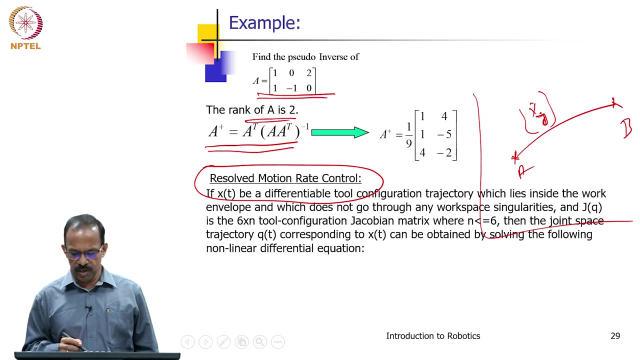 method. So this is known as the Resolved Motion Rate control. you will be learning Cartesian space and I will say that from this point to this point, it should have a particular x dot and y dot. I will say this as x dot and y dot, or I will say it should have a constant. 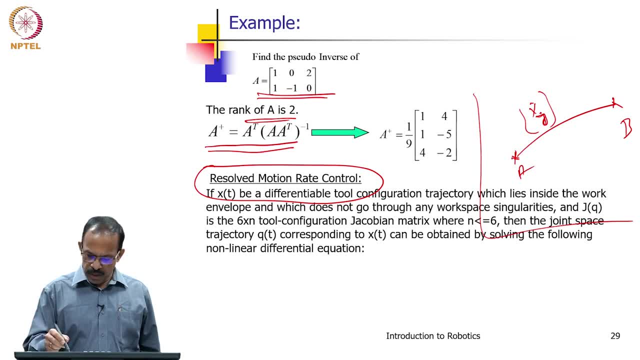 velocity in one thing. So if I have this x dot y dot given, I want to control the robots and then I want to send the commands to the joints to move so that you will get an x dot y dot. So I need to control the joints, So I need 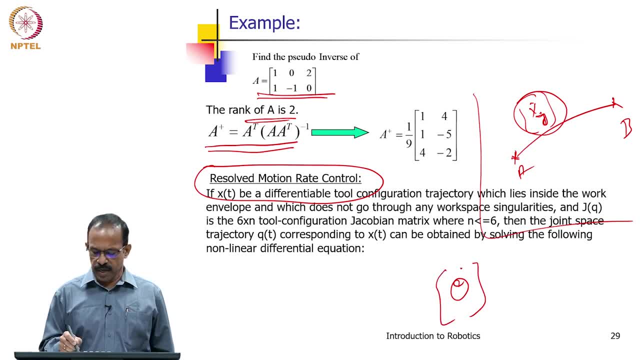 to control the joints, or I would say what should be the joint velocities, and that can actually be obtained by j plus x dot. So I can say that the control, the joint velocities to be calculated based on this, and then I command that velocity, I will be getting the. 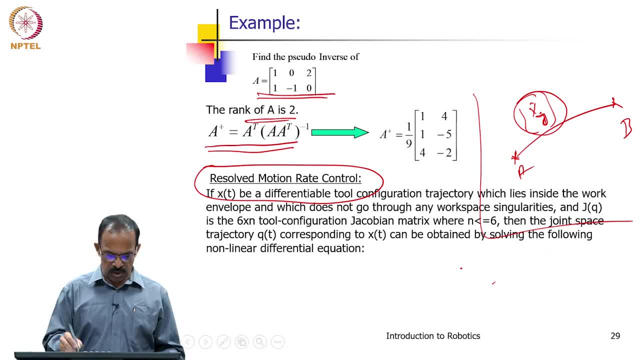 robot motion control and that is known as the resolved motion rate control. So if xt be a differentiable tool configuration trajectory which lies inside the workspace and which does not go through any workspace singularities, and jq is the 6 by n tool configuration jacobian matrix where n is less than or equal to 6..